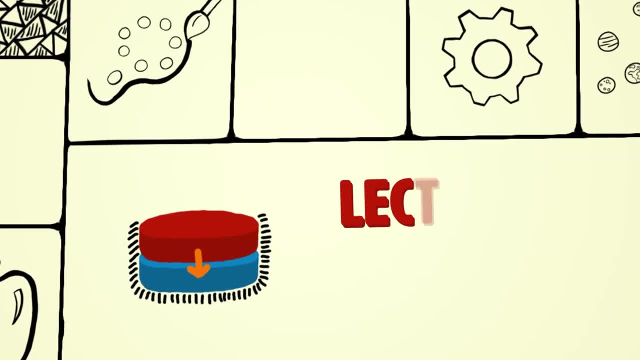 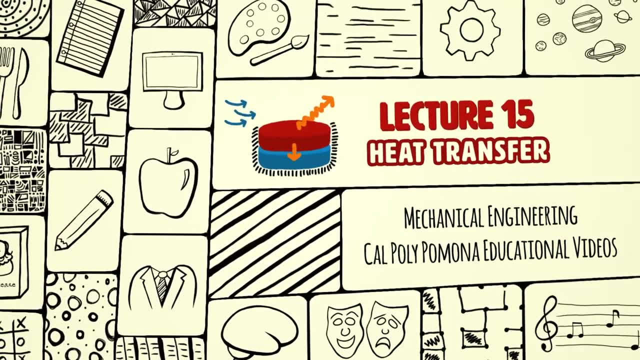 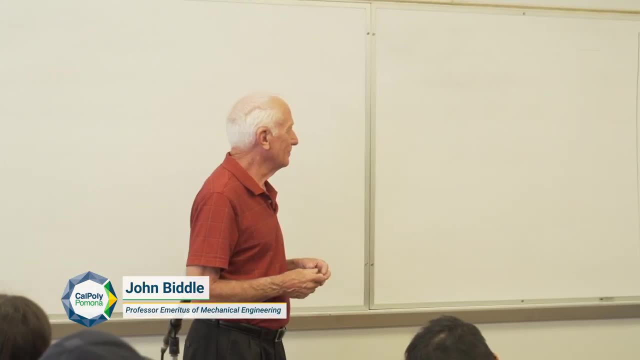 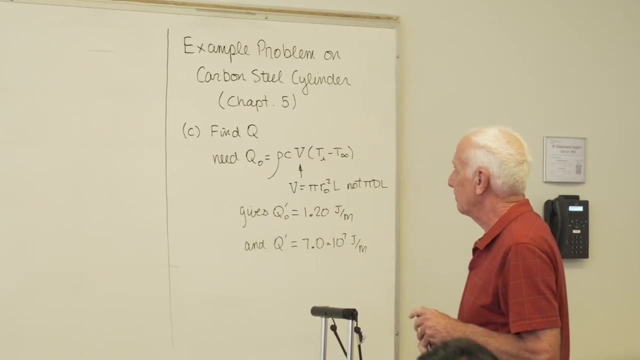 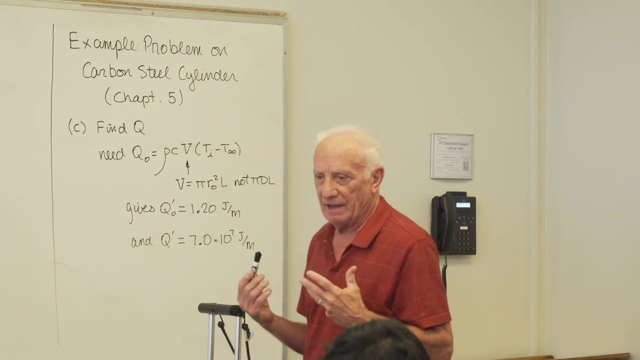 A correction on the class notes. last time We were doing an example problem on carbon steel cylinder transient heat conduction, Chapter 5.. Part C was find out how much energy had been gained by the cylinder after a certain amount of time. This was the equation that we had. 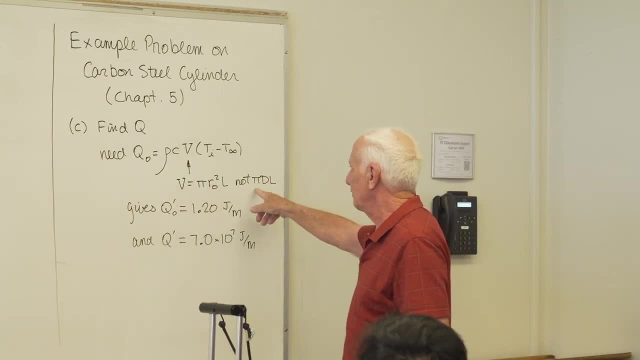 but I didn't put the volume down, I put the surface area down. The volume of that cylinder of course is Pi R squared times L. Make that change in your notes. and here are the two correct answers for Part C of that problem. 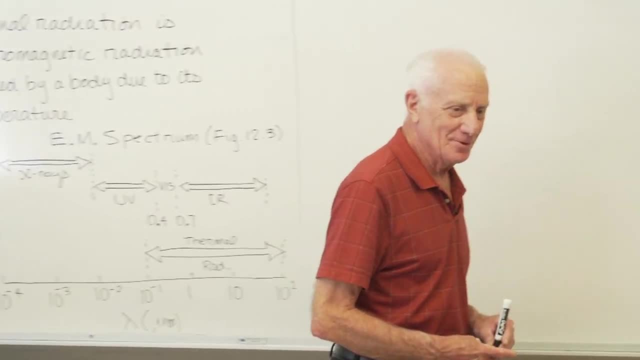 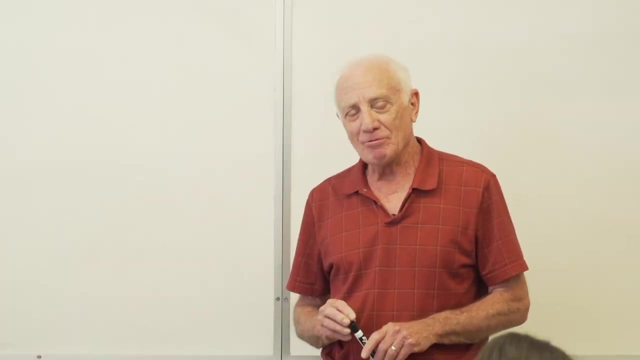 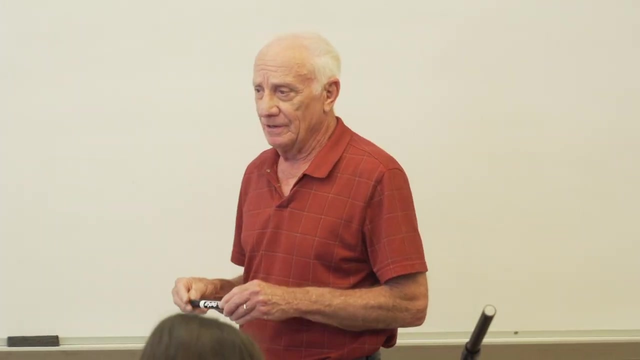 That concludes the four chapters on conduction heat transfer: Chapters 2,, 3,, 4, and 5.. Now we're going to jump to Chapters 12 and 13, radiation heat transfer, and come back in the last third of the course for 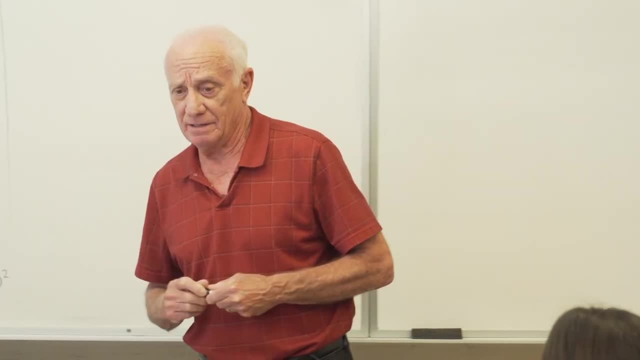 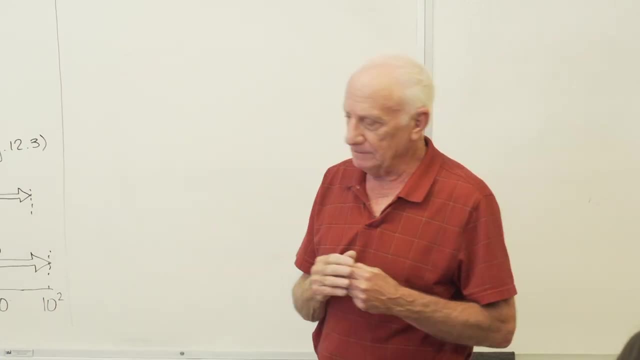 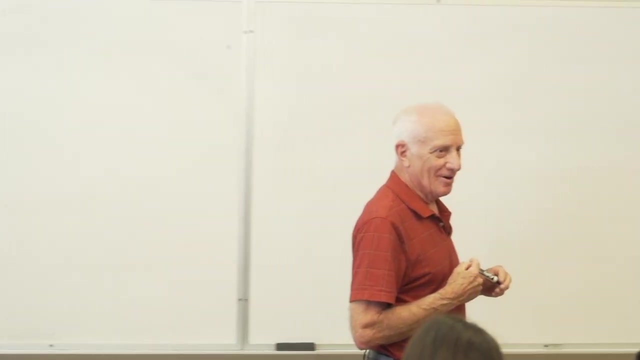 Chapters 6,, 7,, 8, and 9, convection. So we're going to start Chapter 12, radiation heat transfer. Chapter 12 is probably the hardest chapter to read and understand. You've been through that already. You're smiling, I see. 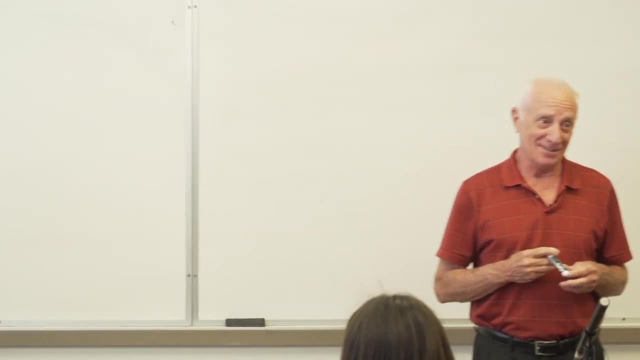 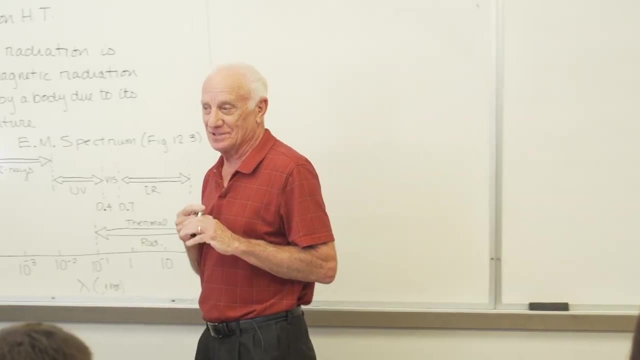 It's a hard chapter to read and understand. So what I'm saying is: take good class notes. I'm going to pick and choose that chapter. what I think is important for this course, Besides the fact of the three modes of heat transfer. 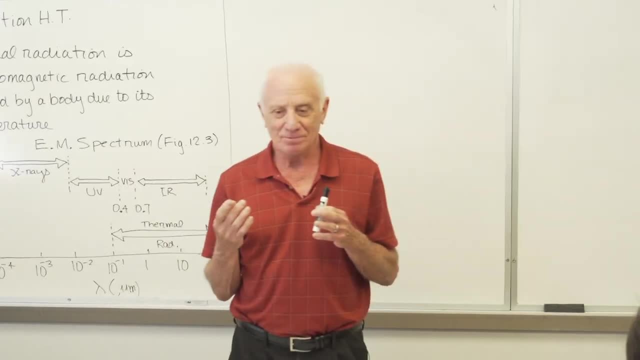 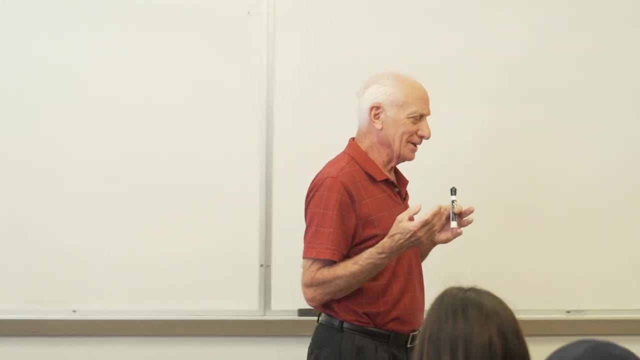 conduction, convection and radiation. radiation is probably the one that you have the least experience with. All people experience conduction all the time and especially convection. Our whole life. what we build a lot of times revolves around convection- heat transfer. 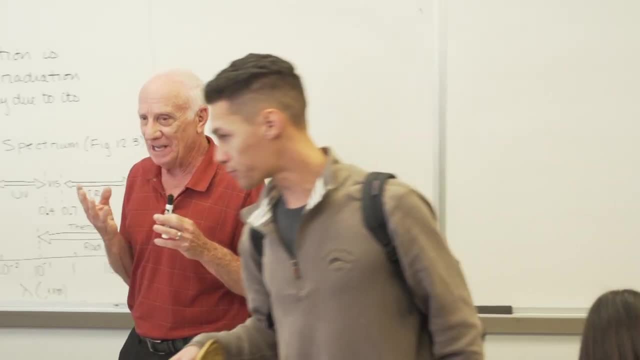 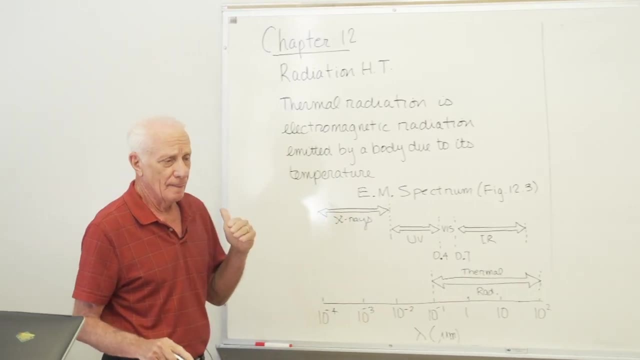 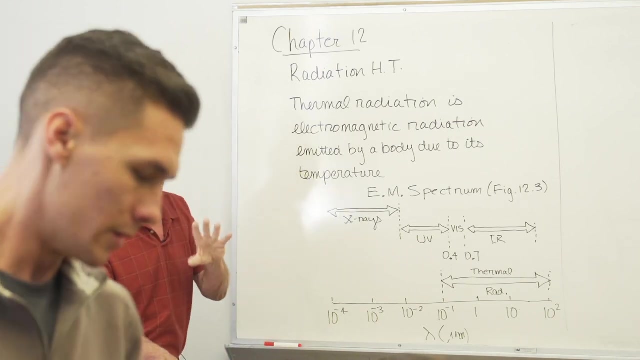 But radiation is something that people don't have a good handle or feel for. So let's first of all define what we mean by thermal radiation. Thermal radiation is the heat transfer part of radiation- Thermal radiation- we're going to consider this to be. 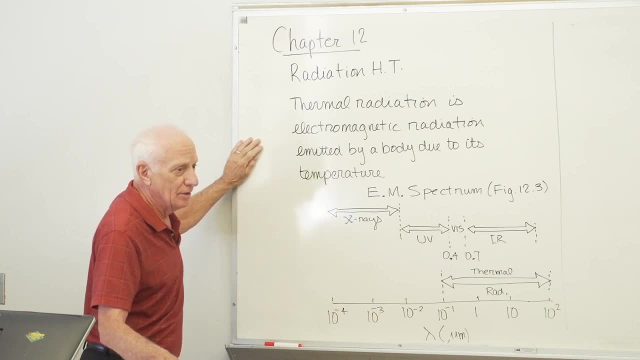 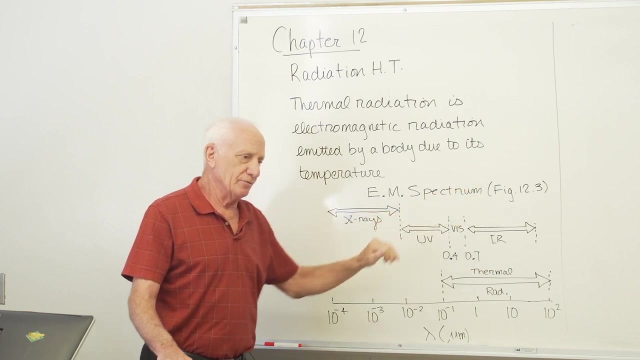 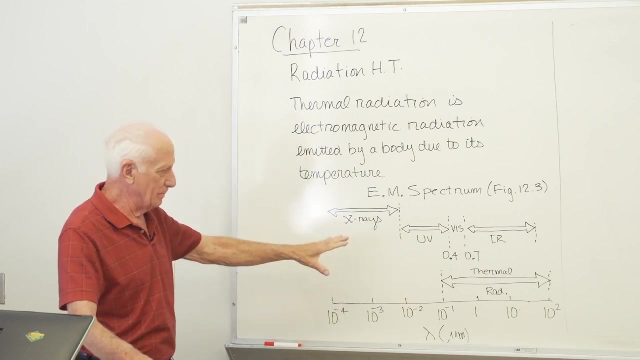 electromagnetic radiation emitted by a body due to its temperature. The two important things there are electromagnetic radiation and it's due to the body's temperature. Electromagnetic spectrum. figure 12.3 in Chapter 12 looks like this. We're plotting different parts of the spectrum versus wavelength. 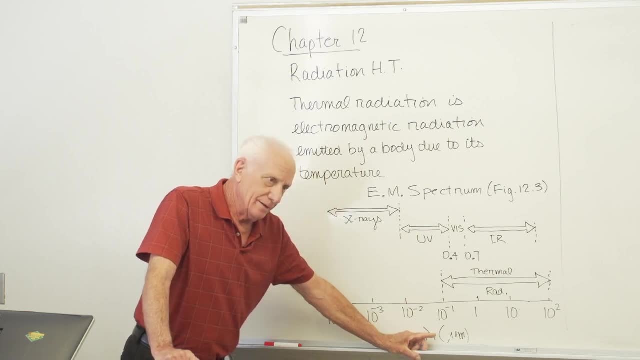 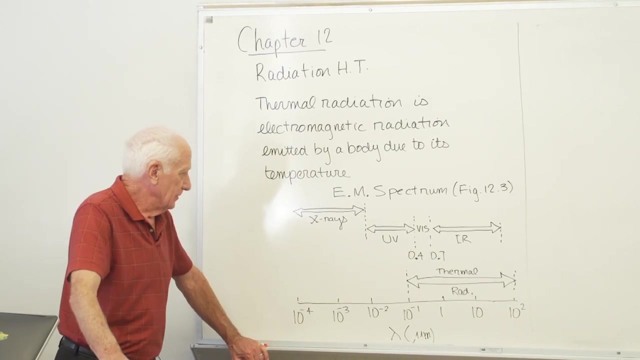 Wavelength down here microns. microns 10 to the minus 4, it's a log scale out to 10 to the 10th 100.. So, first of all, short wavelengths, Just for instance. what's some short wavelengths? 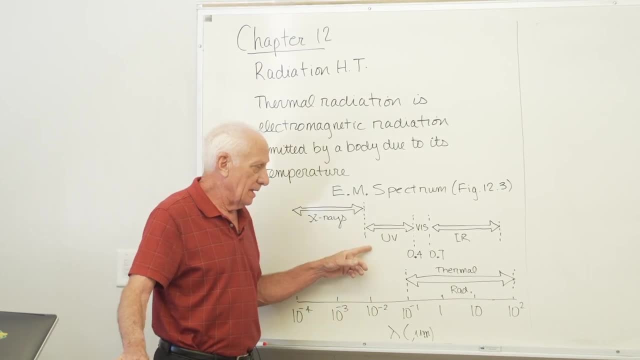 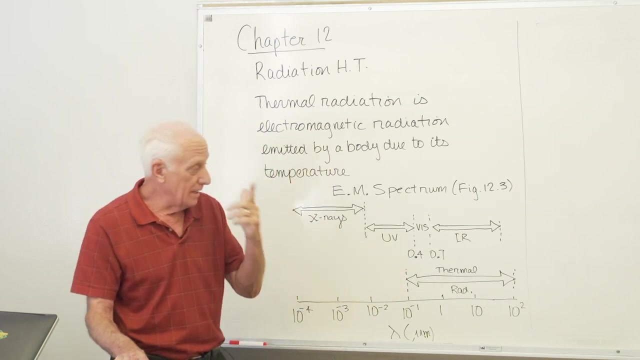 X-rays. How about ultraviolet? Typically in this particular part of the spectrum, part of the chapter ultraviolet, from 0.01 down to 0.4.. Visible spectrum that we see with our eyes: seven-tenths, four-tenths to seven-tenths. 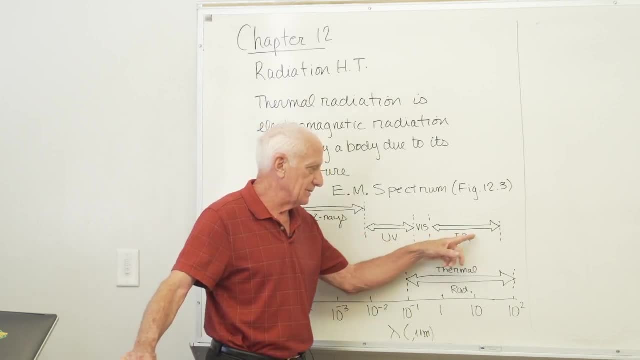 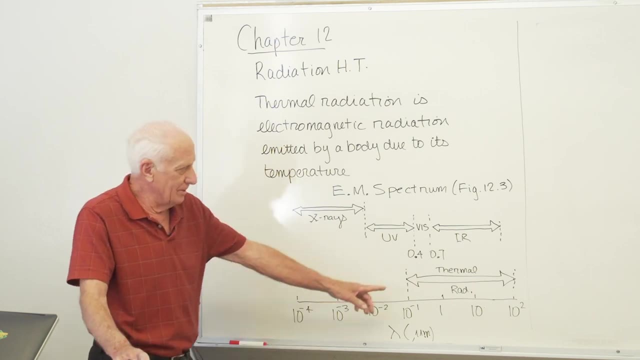 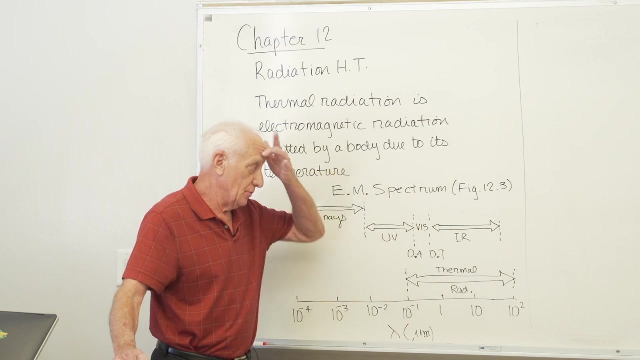 Infrared long wavelengths seven-tenths out to 100.. Where does thermal radiation fit into this? Here's the thermal radiation part of the electromagnetic spectrum. It goes from 0.1 out to 100.. That's what we're looking at. 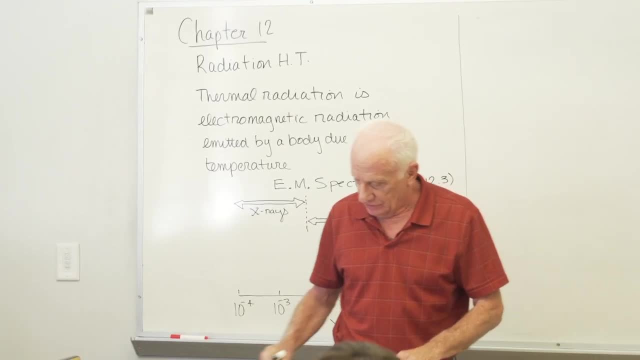 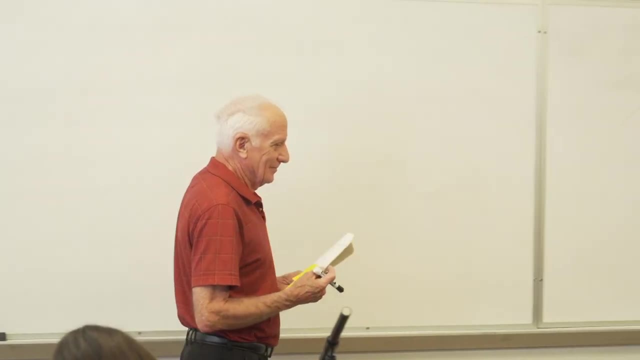 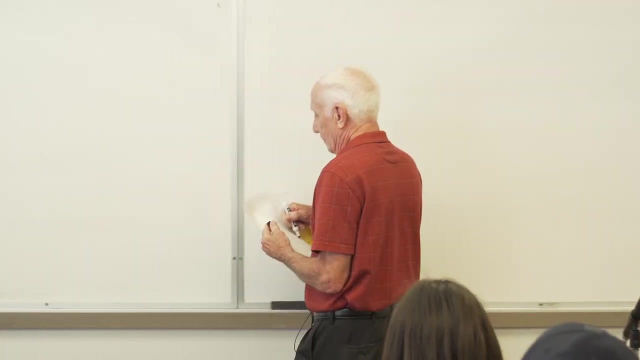 Now we go back to our Chapter 1.. We had a very brief introduction to thermal radiation in Chapter 1.. We talked about the concept of a black body. We'll go back to Chapter 1 and expand on that. So, black body. 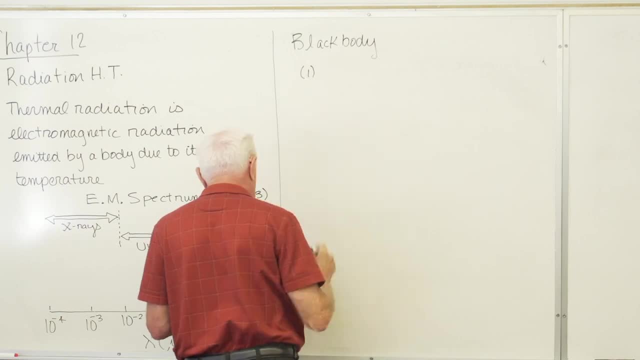 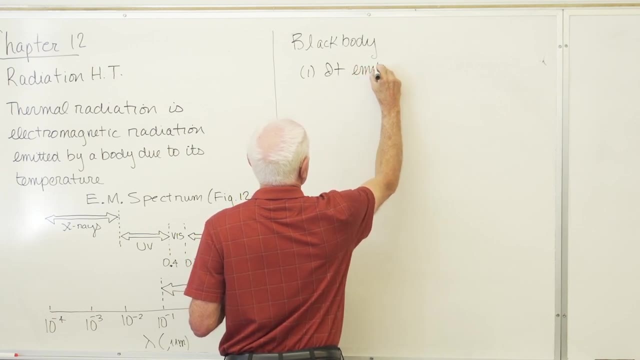 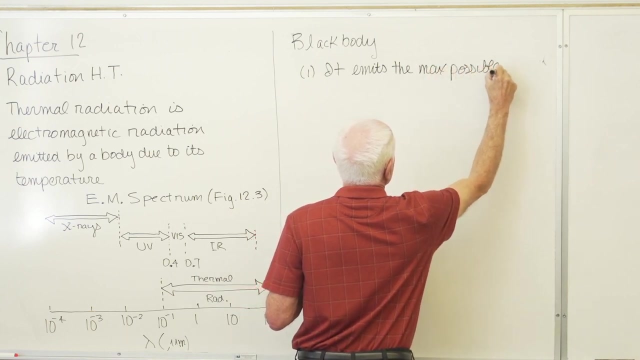 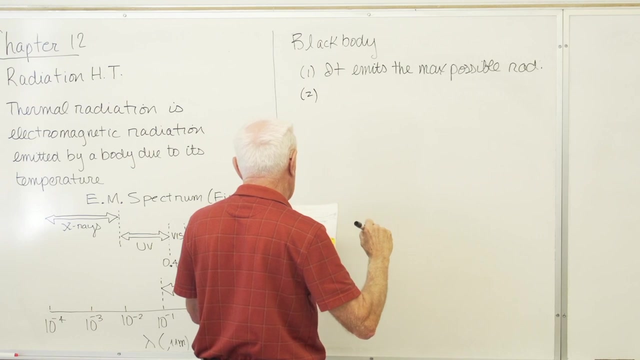 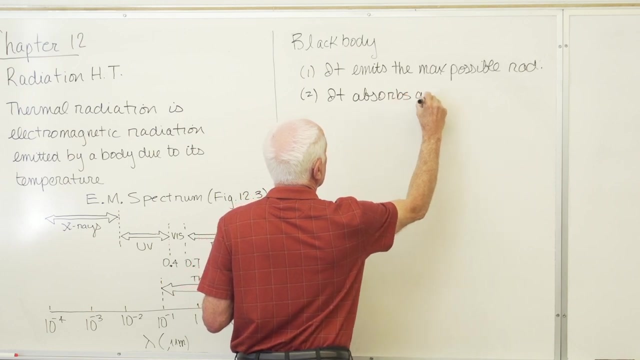 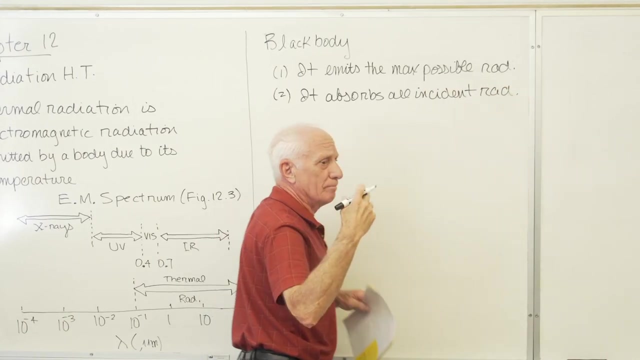 I'm going to put down two important concepts of the black body. It emits the maximum possible radiation. Number 2, it absorbs all incident radiation. There's a number 3 that says it's also a diffused surface, but I don't want to discuss a diffused surface right now. 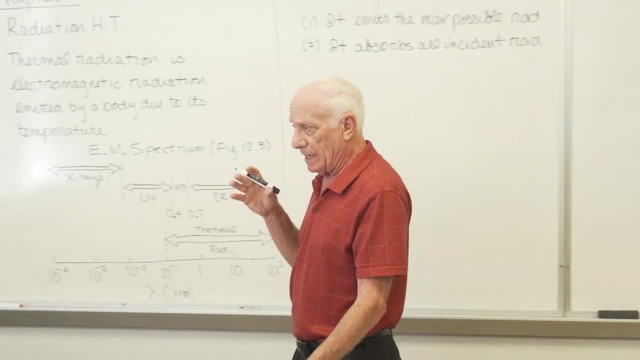 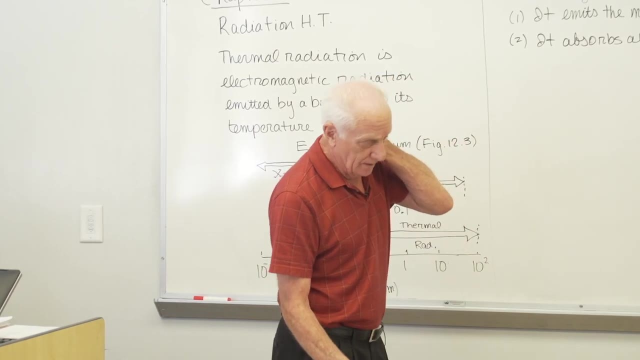 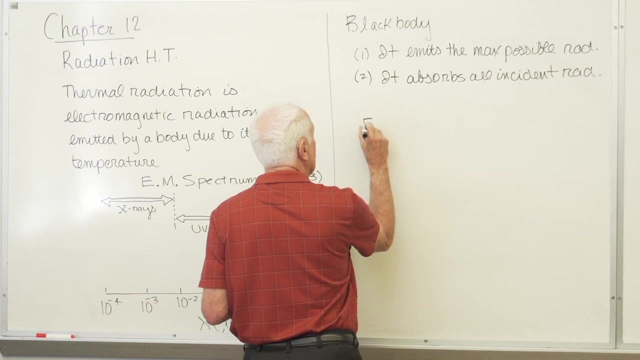 so we'll get back to that later on. But essentially, a black body absorbs all incident radiation and it emits the maximum possible radiation. Now, how is that radiation distributed? Well, it's distributed according to something called the spectral black body emissive power. 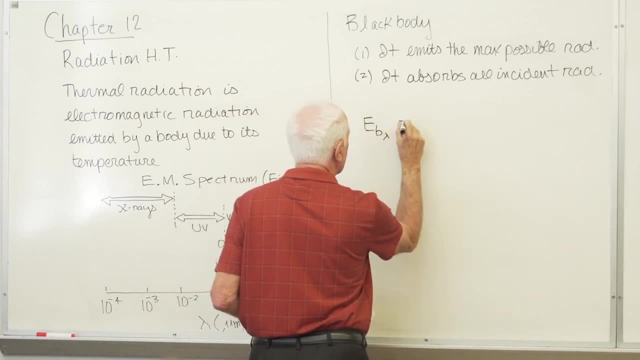 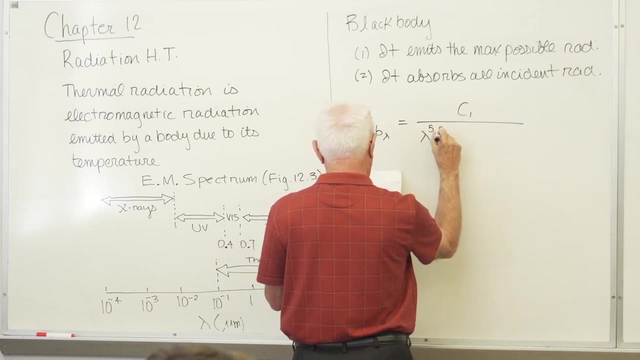 I'll write the equation down first, then I'll define this. So it's obtained E b lambda by dB lambda. Now that's going to be equal to the amount of light that it emits when it's exposed to the surface of the black body. 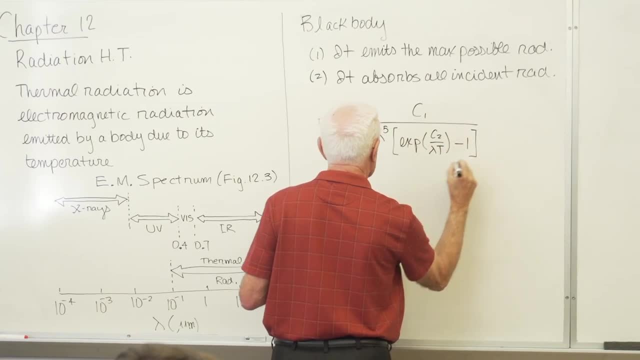 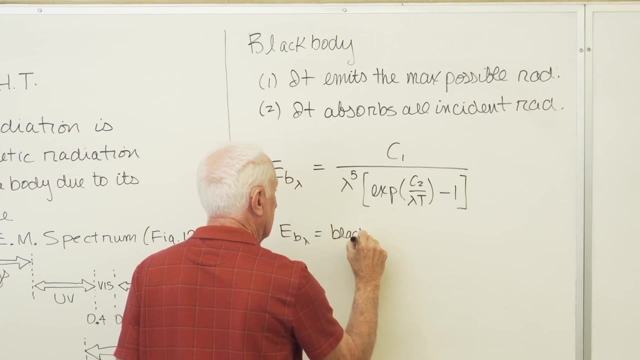 so that's what we're looking at. You can see that when we've dilute theAC2, it actually emits E b lambda, And this is a good idea, because the black body emits radiation. so that means we're going to be able to describe it in terms of tasty. 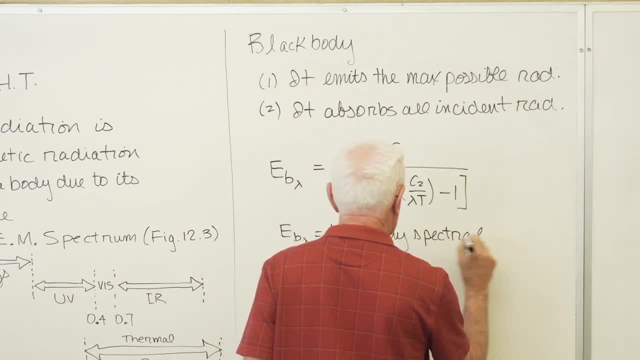 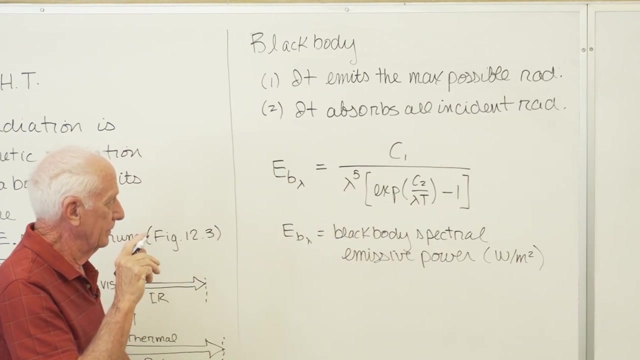 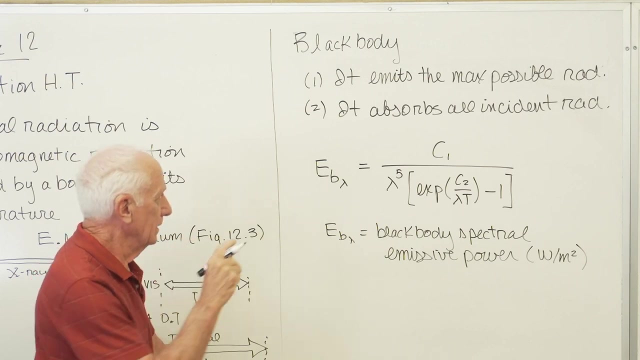 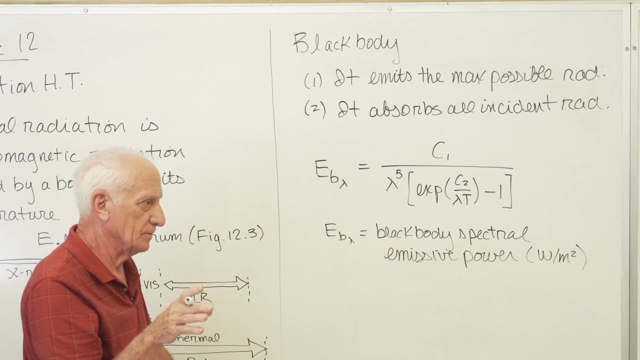 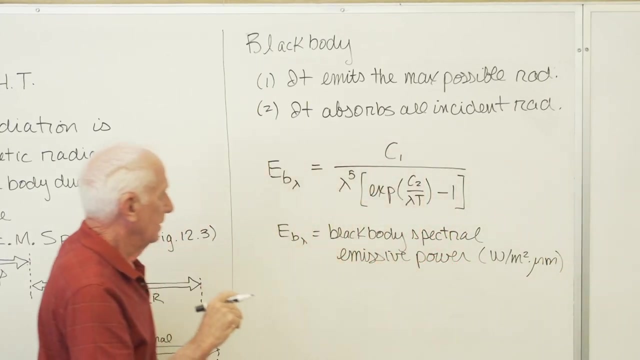 There's two subscripts, There's a B and there's a Lambda Capital E, Chapter 1, stands for emissive power. Units are watts per square meter per micron. here, Of course, B means black body, not a problem. 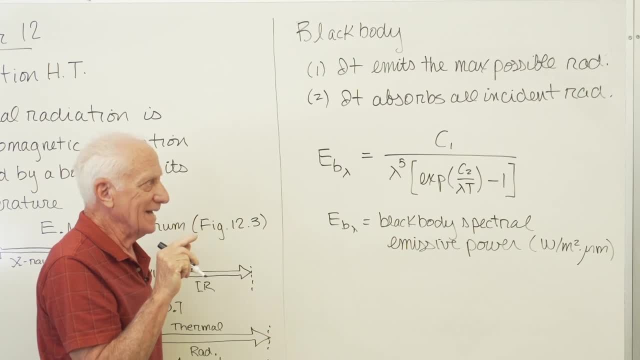 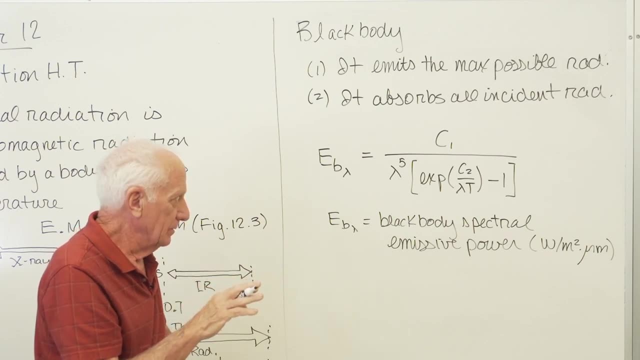 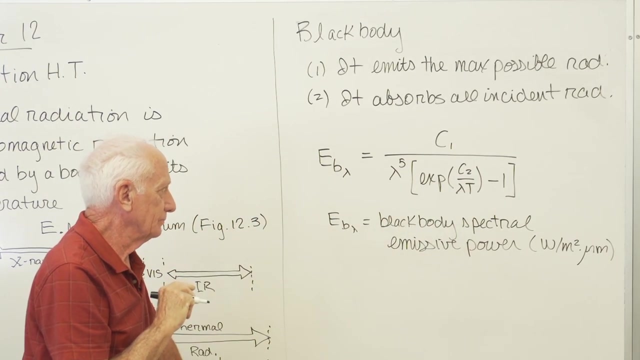 Lambda means at a certain wavelength. That's called spectral. Spectral means wavelength dependent. You have to give me a wavelength right there Lambda in order for me to give you an eB Lambda. It's wavelength dependent. Just a reminder, remember. 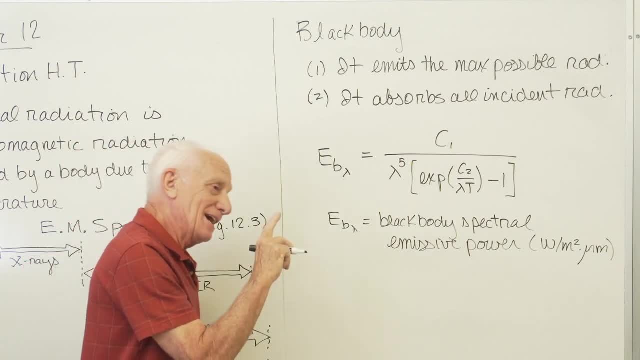 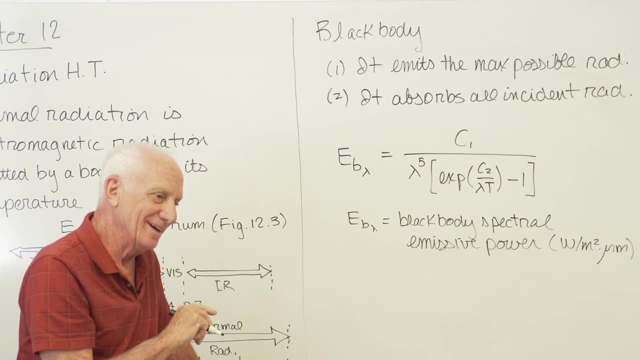 anything to do with radiation. every time we see a temperature has to be at absolute. If we're given the problem in degree C, add 273 degree K, So everything should be converted to absolute right away, before you start the problem, Otherwise you might end up making. 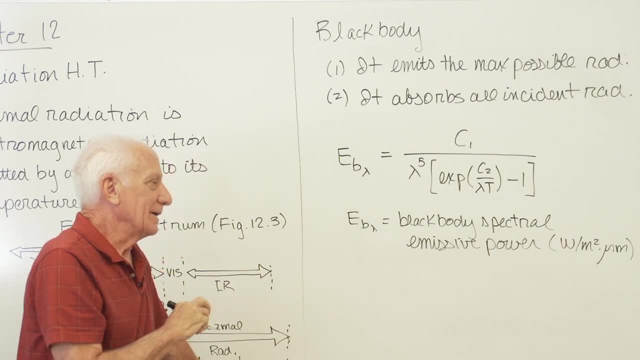 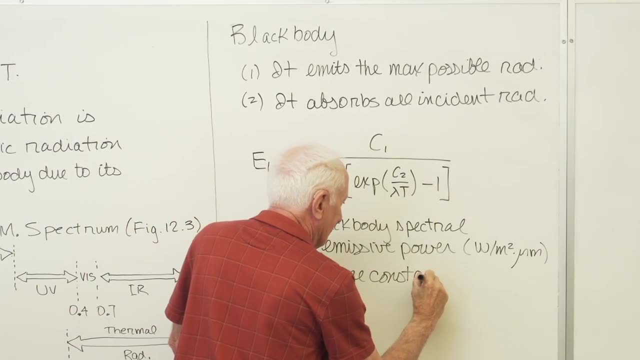 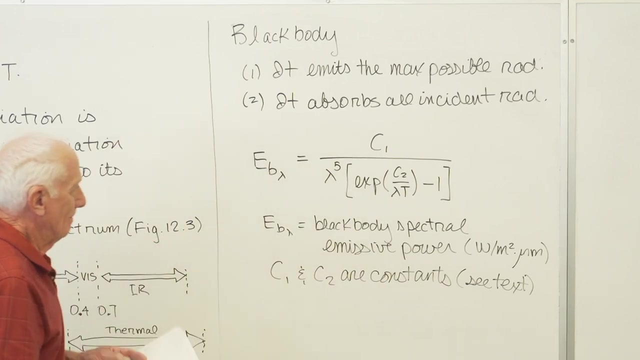 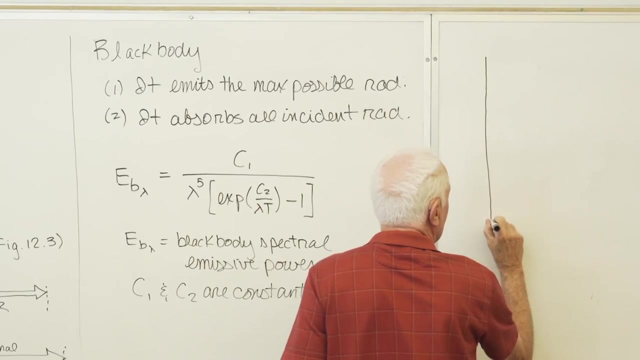 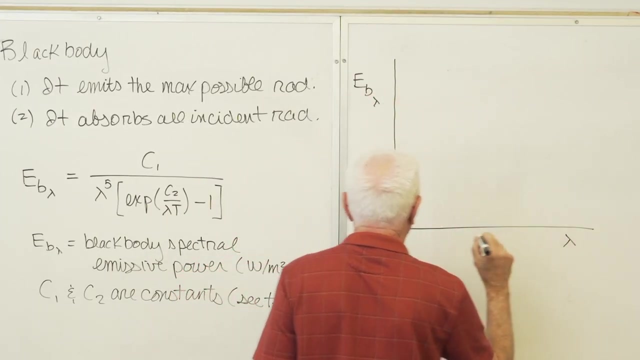 a silly mistake. Okay, C1 and C2 are constants- See the text for values. So we can plot this. We can plot eB Lambda versus Lambda. I'm going to pick a certain temperature. Oh, I don't know. 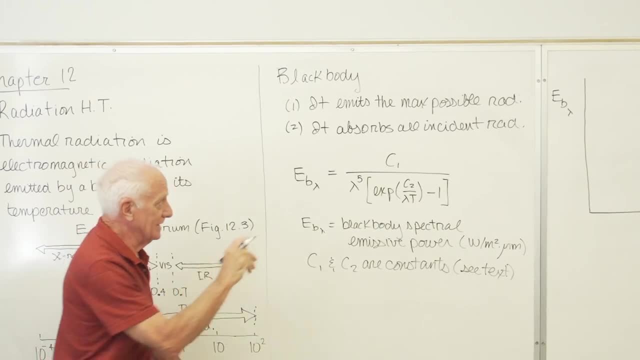 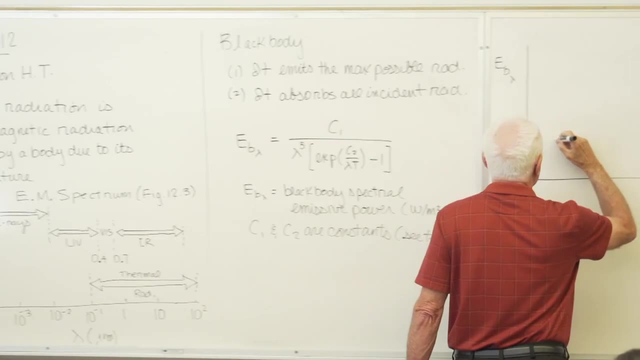 I'll say T is 1,000 Kelvin. Now, if I say T is 1,000 Kelvin, I'm going to plot eB, Lambda versus Lambda. The shape of the curve looks something like this: That's at a temperature T1,. let's say: 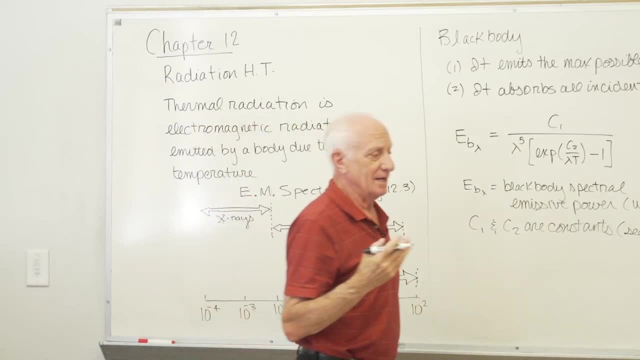 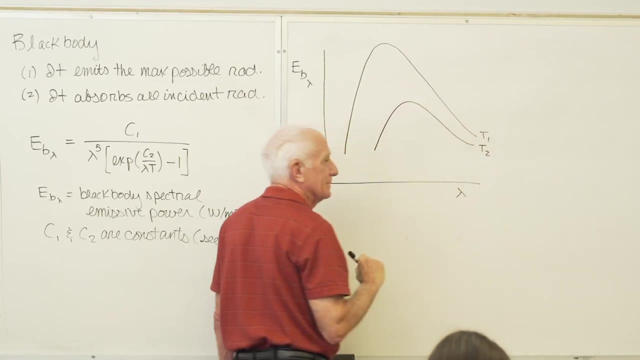 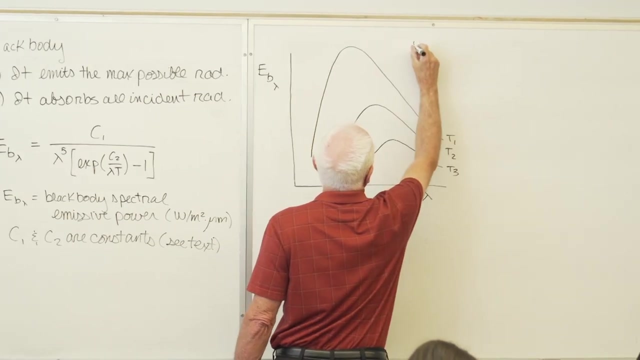 Now I'll choose a different temperature. Oh, let's say, 500 Kelvin Curve Curve looks like this. Let's say, 300 Kelvin Curve looks like this: where T1 is greater than T2 is greater than T3.. 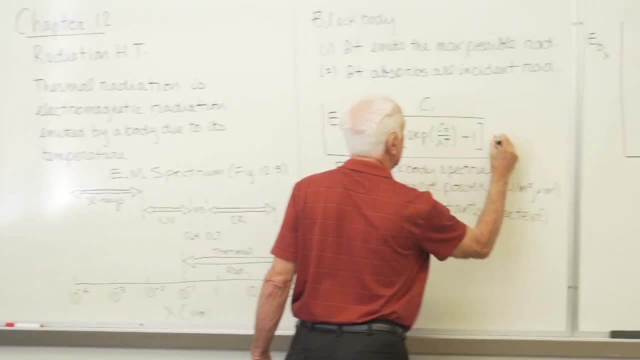 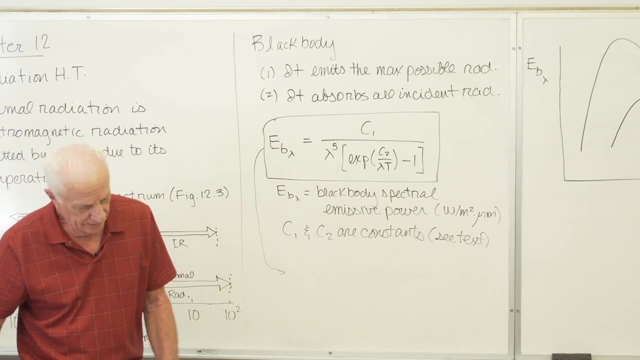 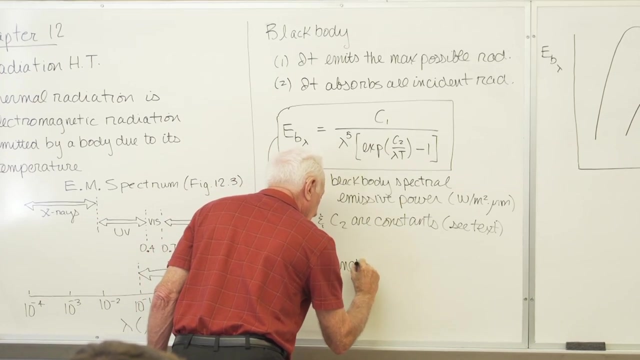 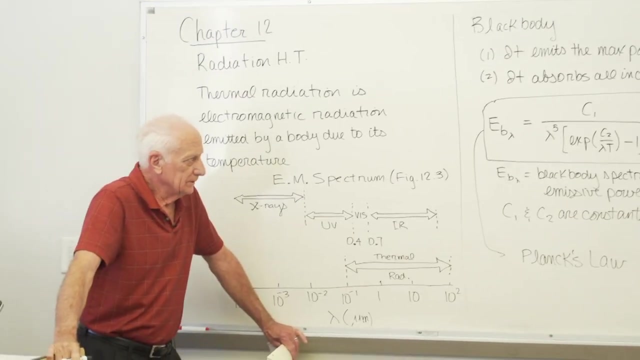 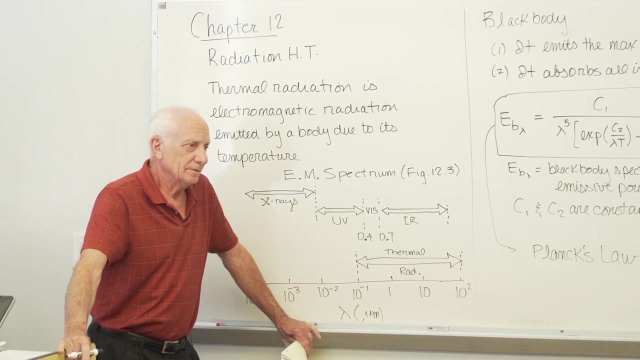 I'm going to box this guy in. Oh, by the way. Okay, Any equations? give it a name: Planck's Law, Planck's Law. Now I notice the shape of those curves. Every curve seems to go down. 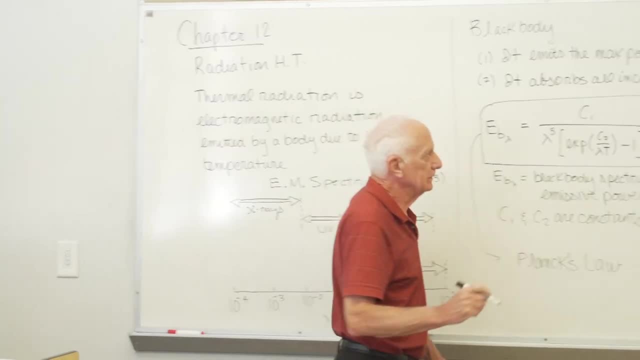 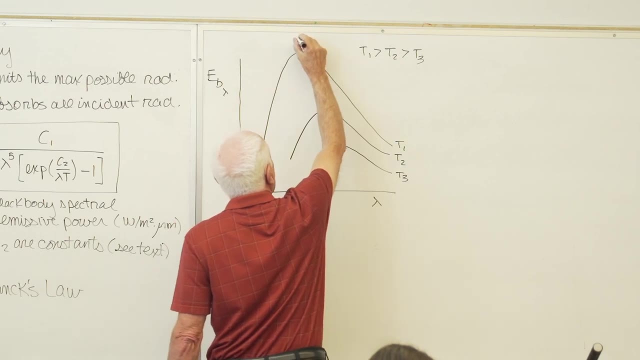 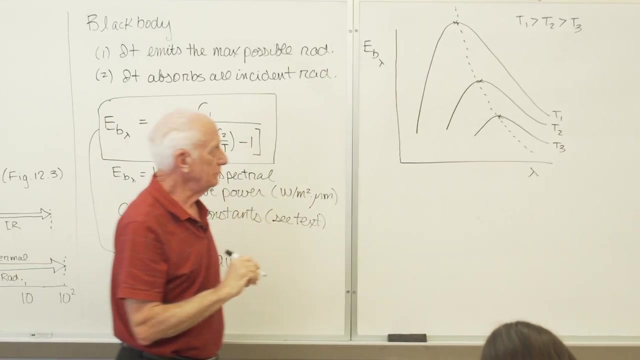 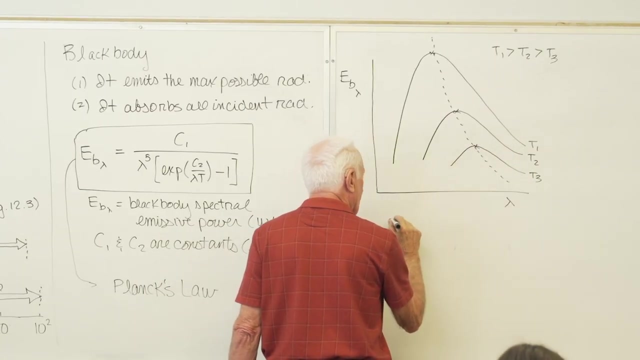 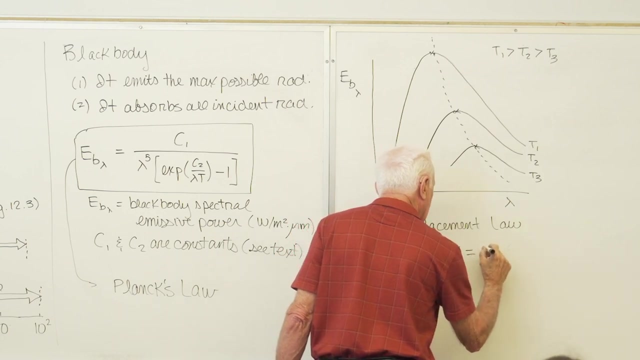 Seems to go through a maximum. Okay, Here here, here, Now I can connect those maximums with a line. Looks like that, the dashed line. If I do that, then I get what's called the displacement law, Which is lambda. max T equals a constant C3. 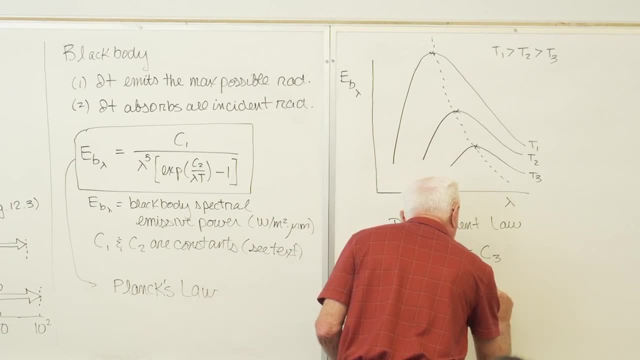 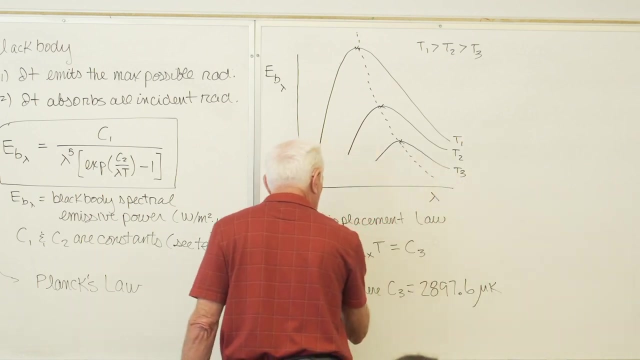 in SI. Okay, Let's get the distributive. This is a way. This is a way of getting the distributive Okay. So all the numbers are in there. All the numbers are in there: 28.97.6.. 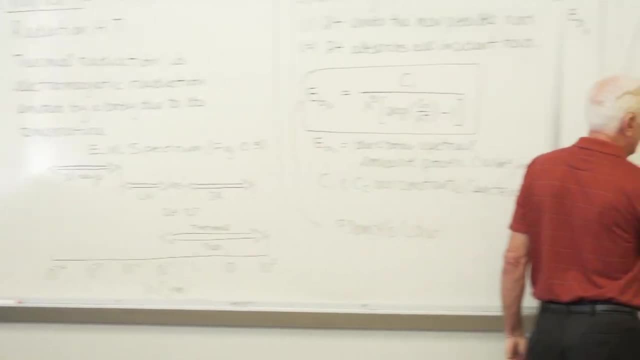 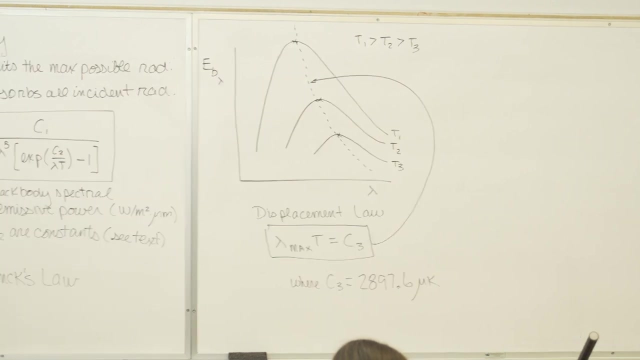 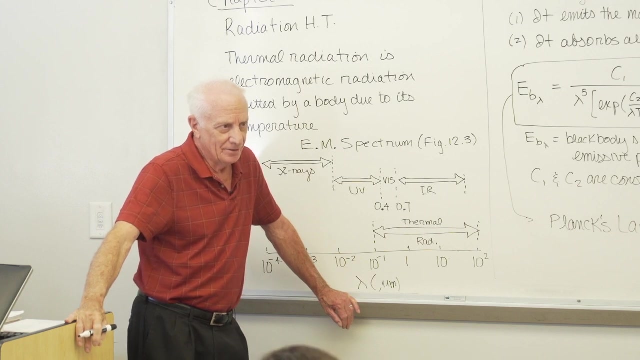 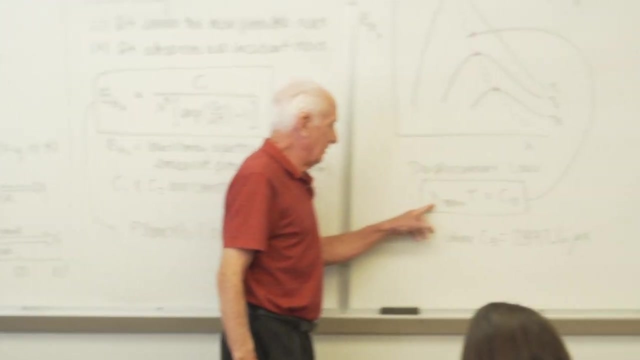 So that equation is the equation of that dash line right there. Now don't get confused by the subscript maximum. That has nothing to do with the maximum wavelength. You don't even say it. Here's what you say. This is the wavelength at which 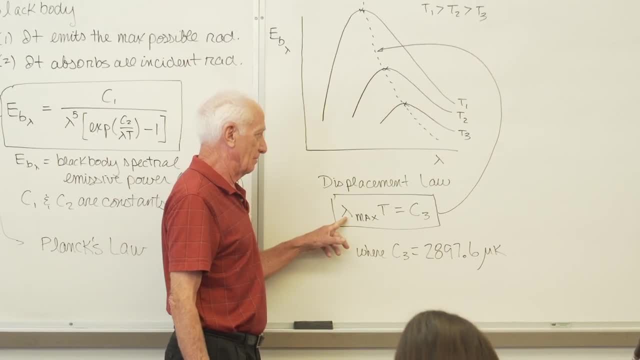 the black-body spectral emissive power goes through a maximum. This is a wavelength where- give me a temperature. I'll give you a wavelength where that curve goes through a maximum. If the temperature is T1, this equation gives me what Go straight down here. 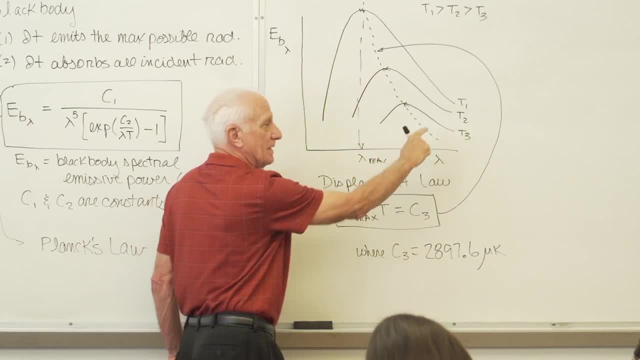 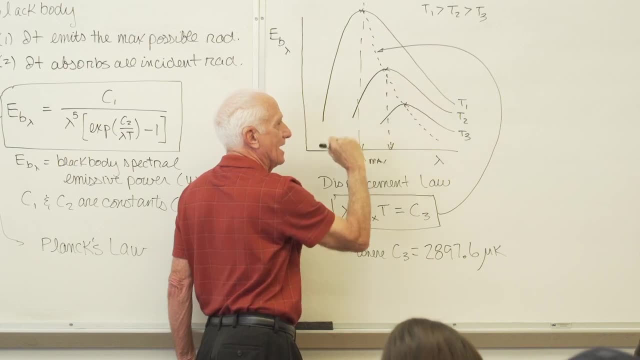 that gives me that value which I call Lambda max. If temperature is T2, put T2 in here. That'll give me where that equation goes through a maximum and so on. That's what it means. It's the wavelength at which 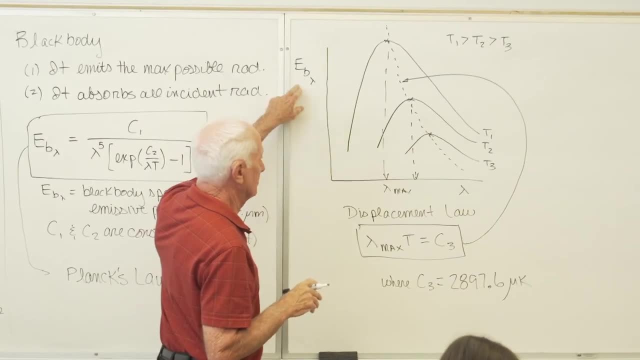 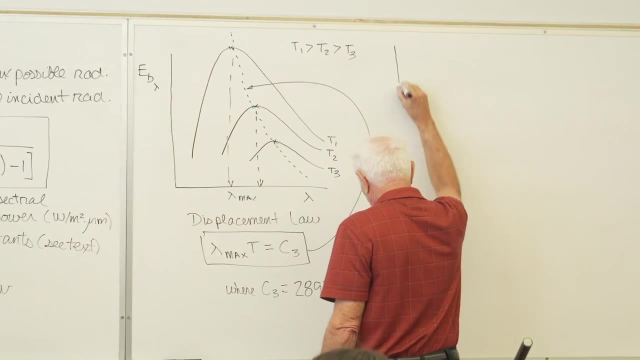 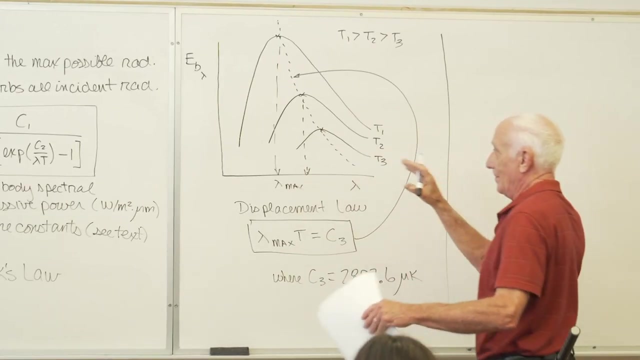 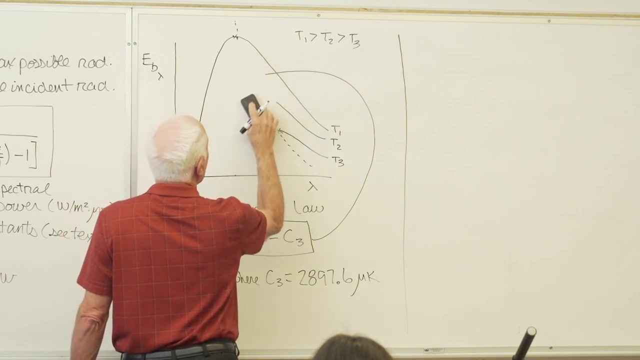 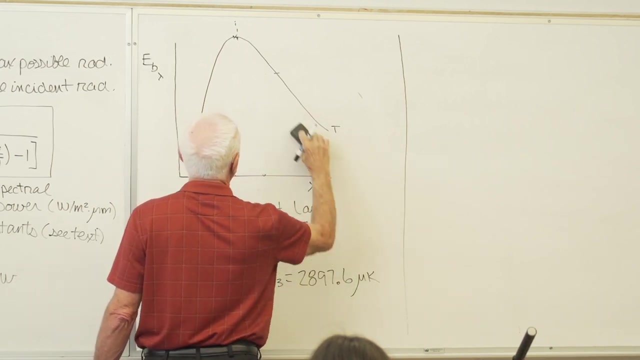 the black-body spectral emissive power goes through a maximum. Now we're going to integrate over the whole curve. I'm going to leave that out. I'm going to leave that guy up there for you. Okay, I want to find the area under that curve. 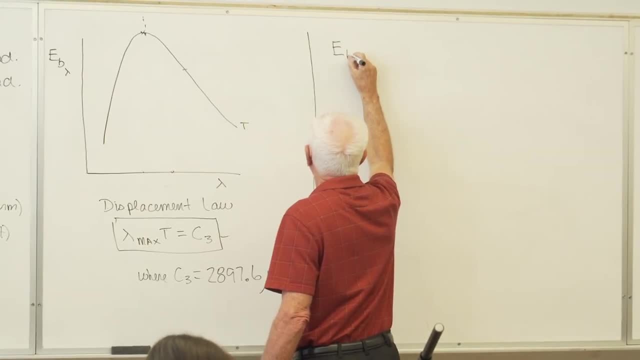 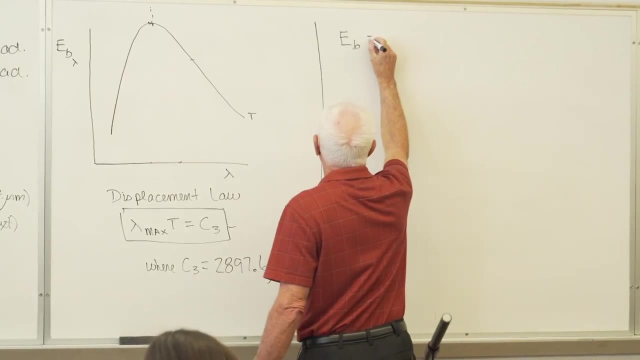 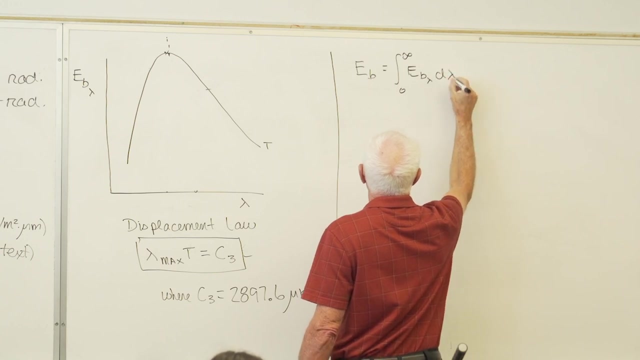 I want the emissive power Eb. I don't want the Lambda on it, I want the total emissive power. I integrate this guy. Let me see any of them: One, two, three, four, five, six, eight. 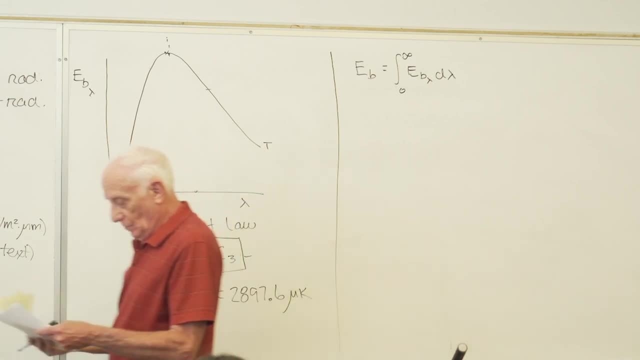 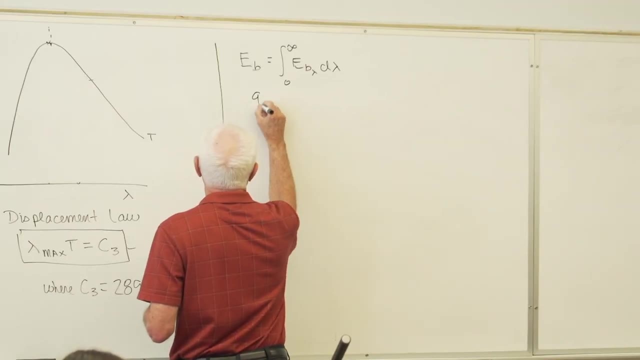 Let it go to this other curve, emax Привет Health, and look at that base that It's very black here, Yes, just boxes up, it's very white. You know it's the Southern Chambers field. Here's what a fill method looks like. 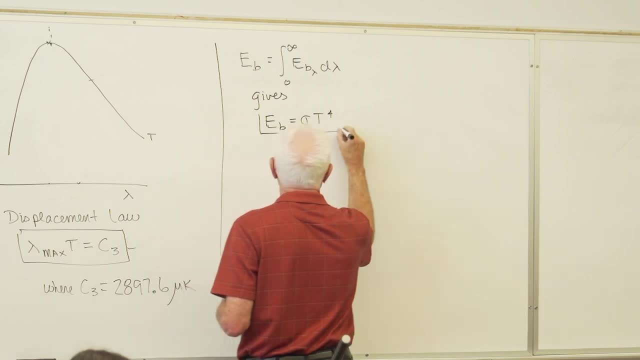 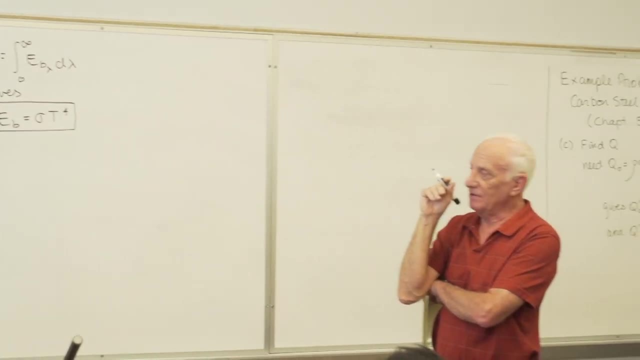 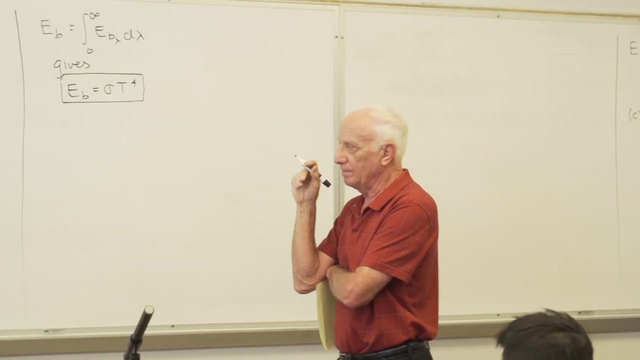 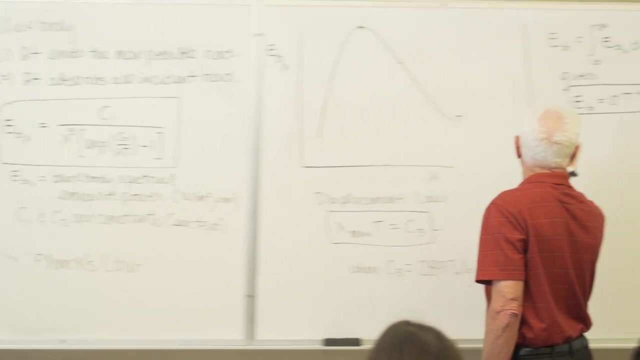 I'm going to form an idea to keep simply as I do. Integrated over all wavelengths, the emissive power becomes a constant sigma times the absolute temperature raised to the fourth power, You think, wow, you integrate this complex expression here and that's what you get. 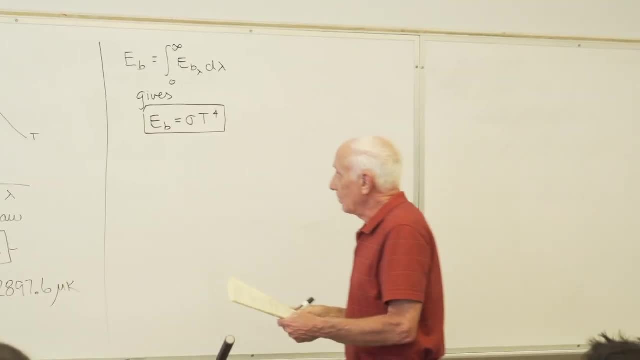 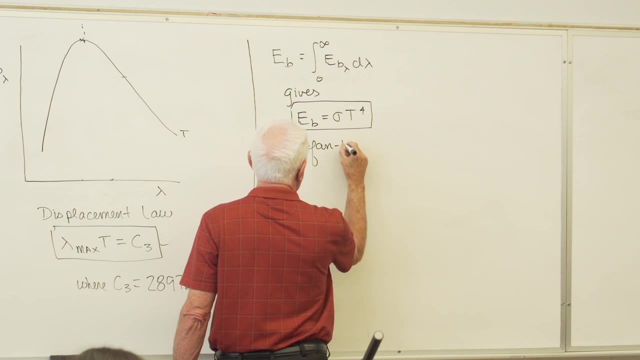 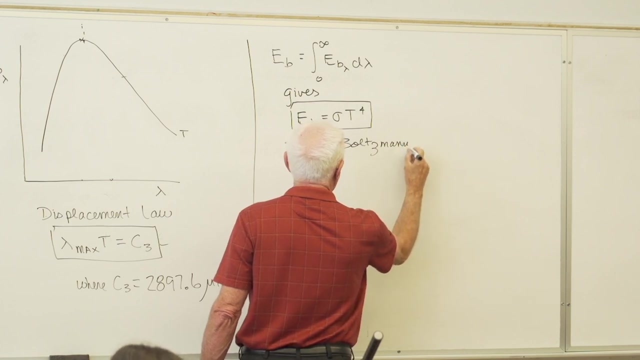 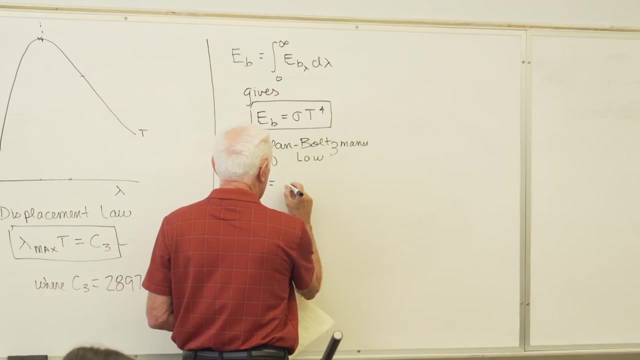 Yeah, that's what you get And of course that's Chapter 1.. So now we have Chapter 1, Stefan-Boltzmann law. Yes, Is the C3 from a chart or is that one value? I'm sorry, say again. 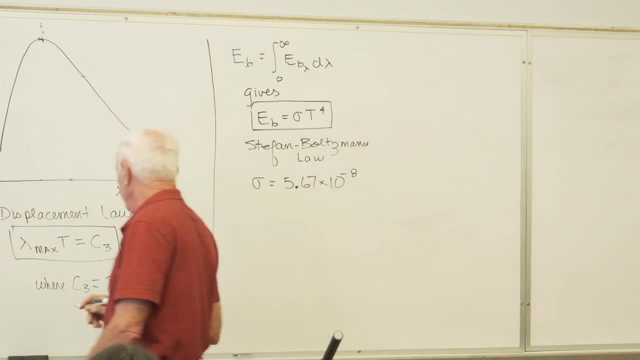 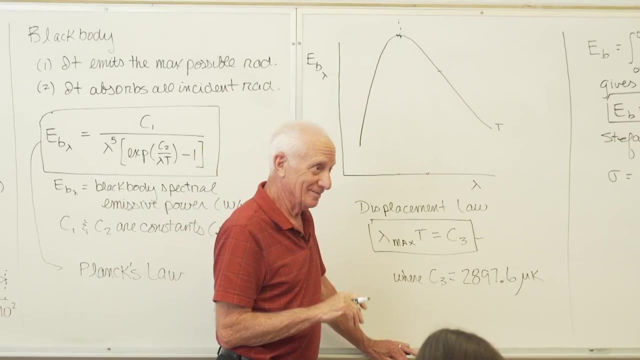 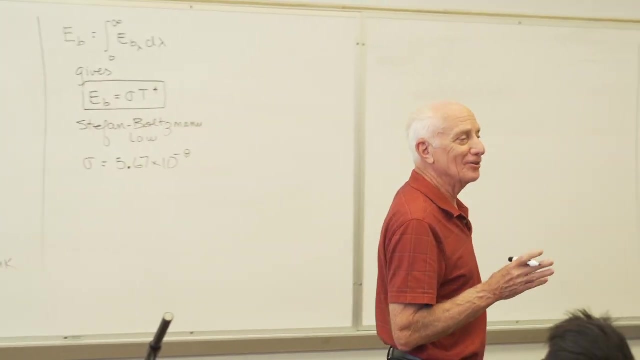 Is C3 from a chart? No, It's in the textbook. It's not a chart, though. Yeah, Yeah, Is that okay? Are there more than that value? There's one in English engineering too, which we don't care about right now. 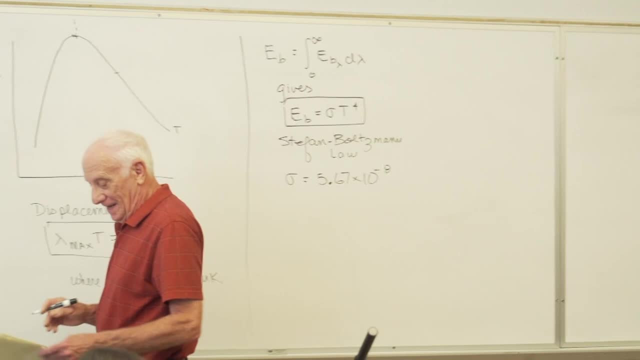 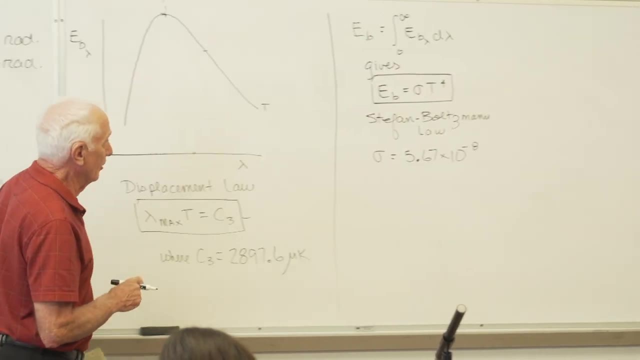 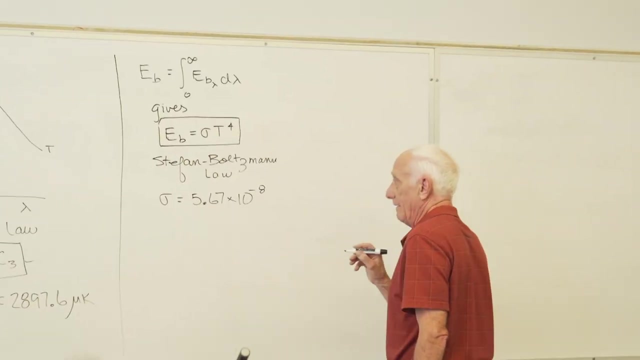 but it's in the book. Yeah, Yeah, Thank you. So that is what we have. we integrate over the whole area. Now we can also say what if we don't want to integrate over the whole area, but we just want to integrate? 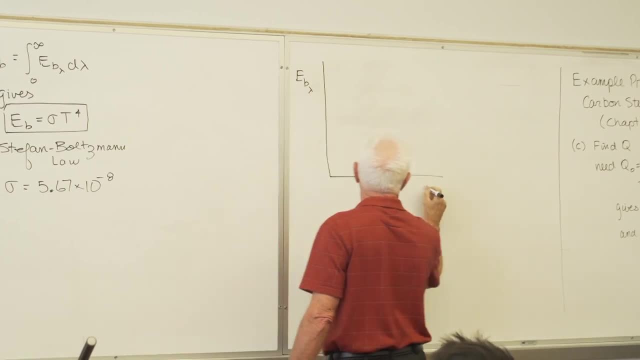 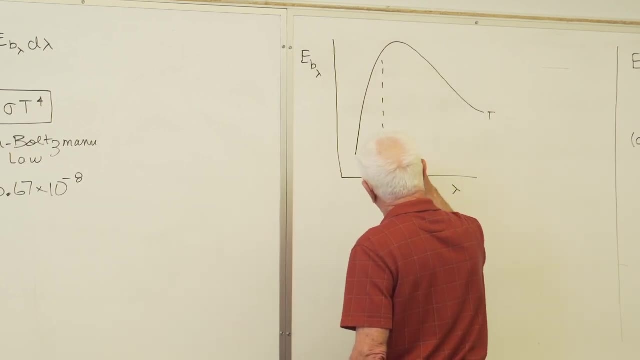 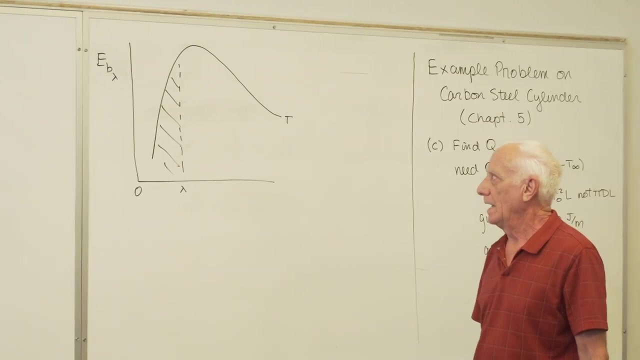 over part of the area. So here's the curve for a certain temperature T, And I want to find out how much energy goes from zero to here. That Lambda can be any value. I don't want to confuse things there. Okay, That area, right there. 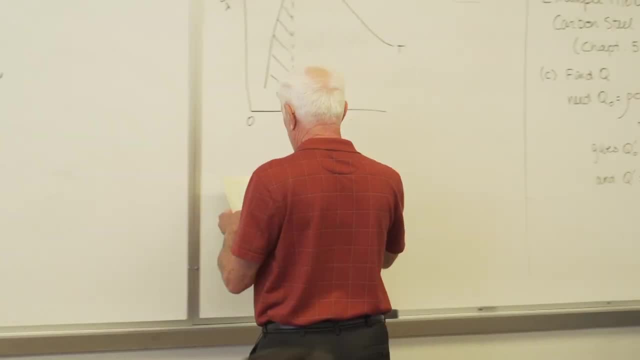 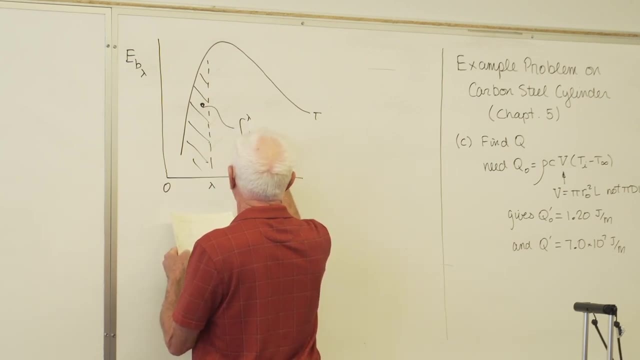 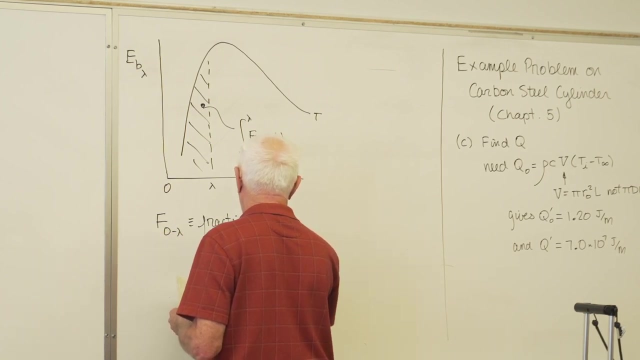 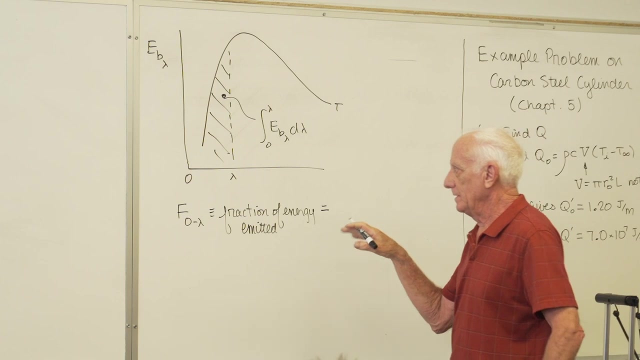 All right, So that area, right there is. this integral, from zero to Lambda E b, Lambda d, Lambda F stands for fraction. I'm going to write an expression for the fraction of energy, this area divided by the total area, That's the fraction. 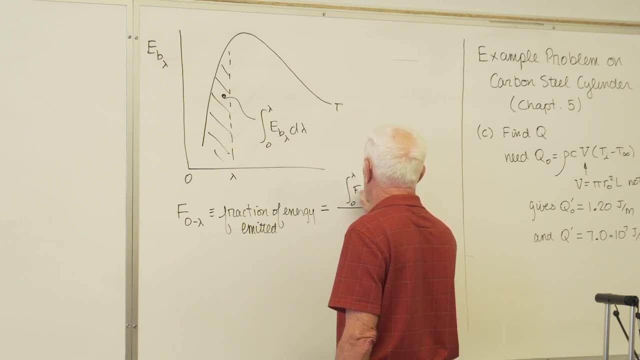 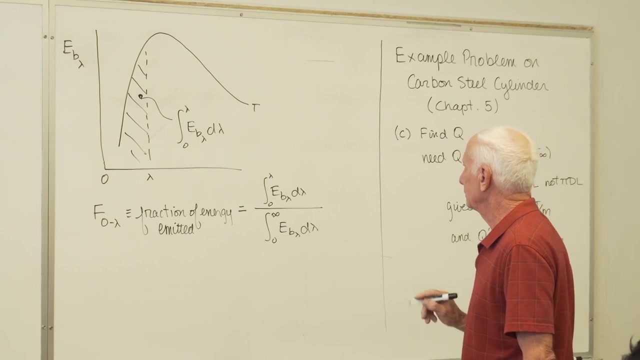 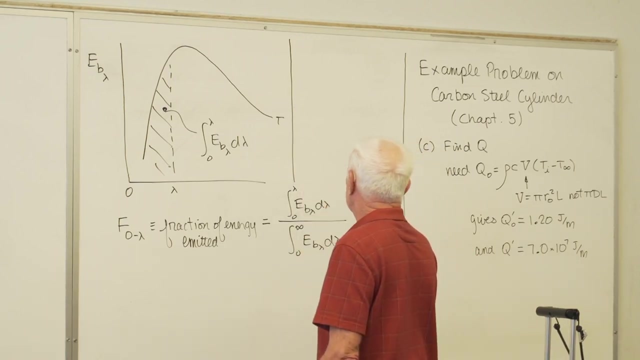 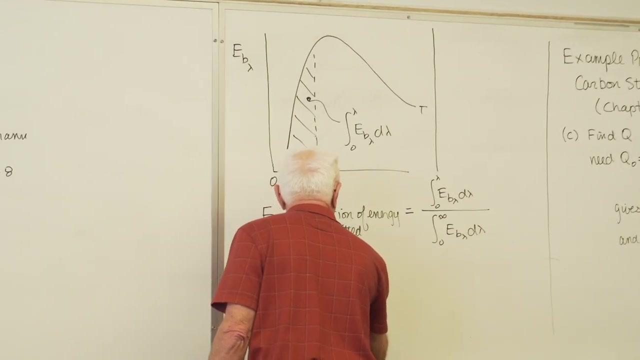 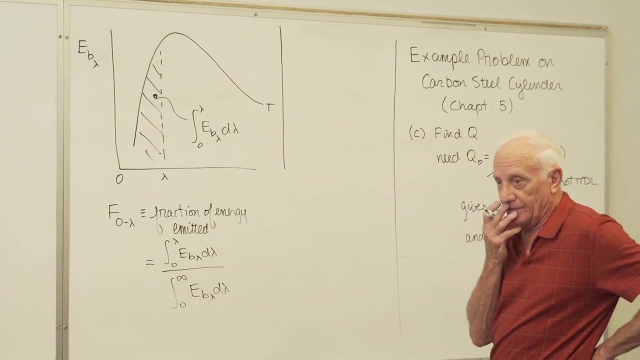 So integral zero to Lambda E b Lambda d Lambda, divided by integral zero to infinity: E b Lambda d Lambda. I'm going to save some space here and put that down here. I need more space And that gives me the fraction. 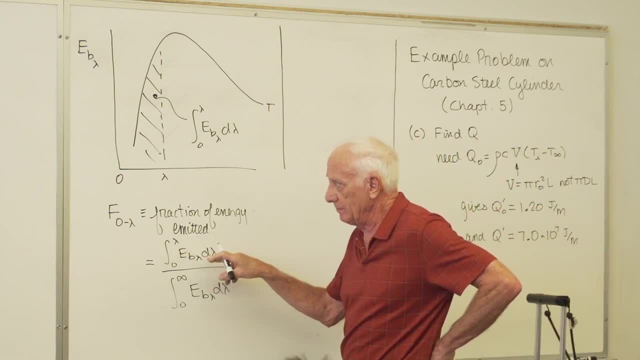 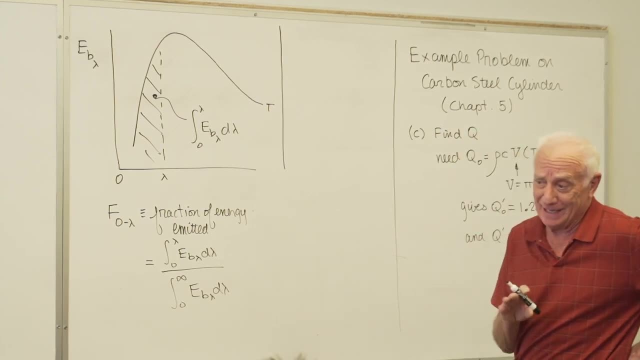 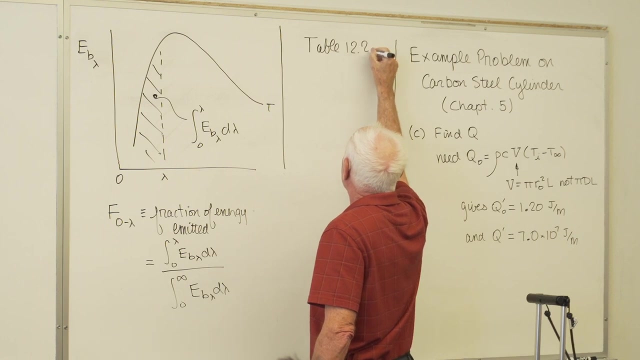 Now what you have to integrate from zero to some Lambda to do that. Well, the book gives you the results that have been done for you, So luckily you don't need to do any integration. Table 12.2.. Table 12.2 gives you one column titled Lambda t. 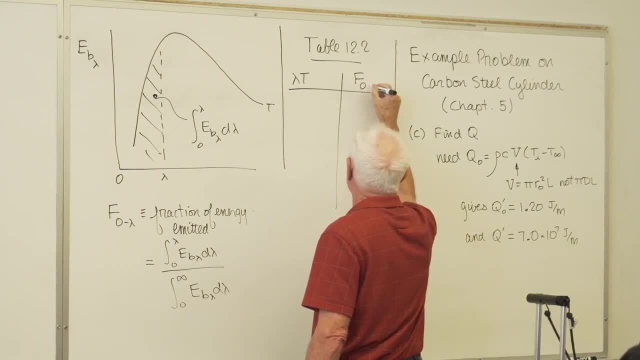 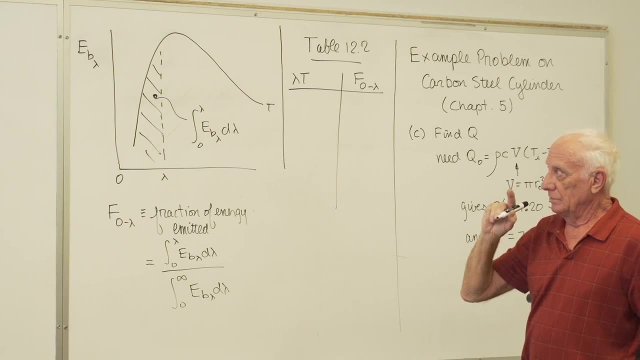 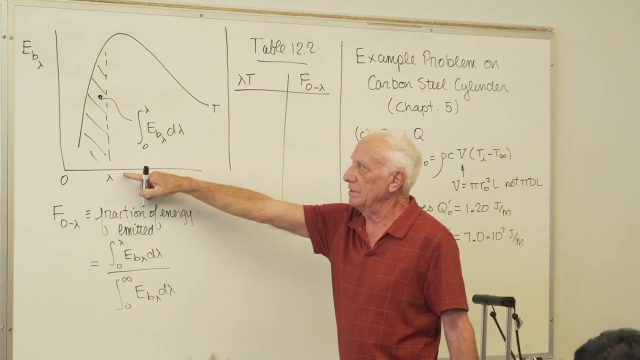 the other column is titled F zero to Lambda. That's this guy here, So left-hand column. take the wavelength Lambda in my picture, multiply it. multiply it by the temperature of the emitting surface absolute. go here, find that value and read off: F zero to Lambda. 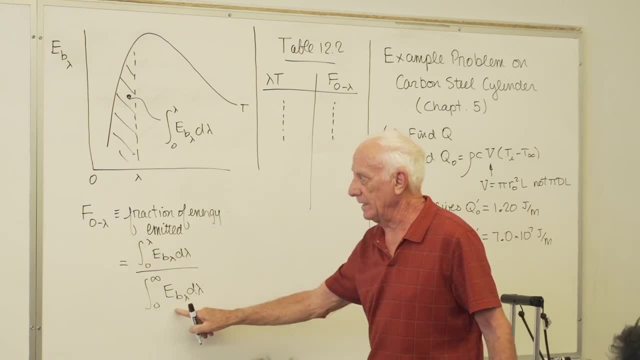 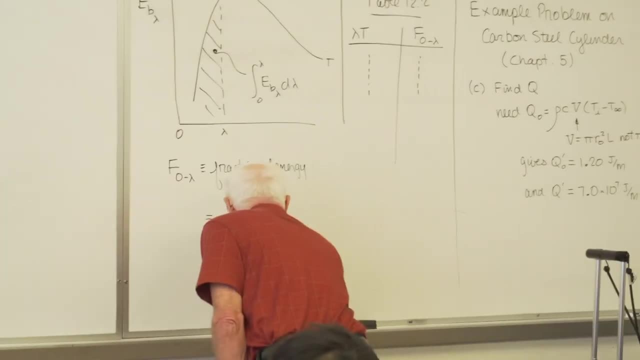 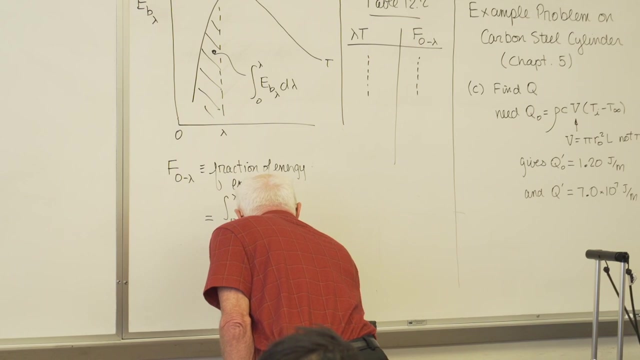 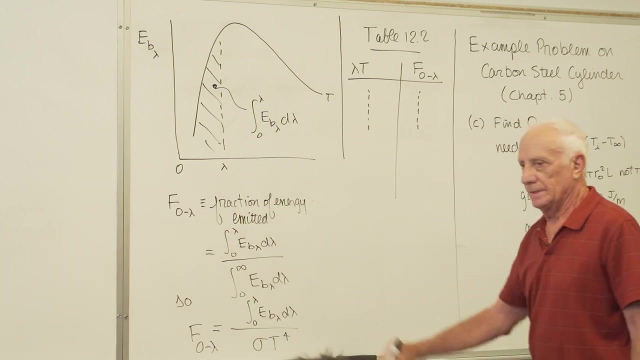 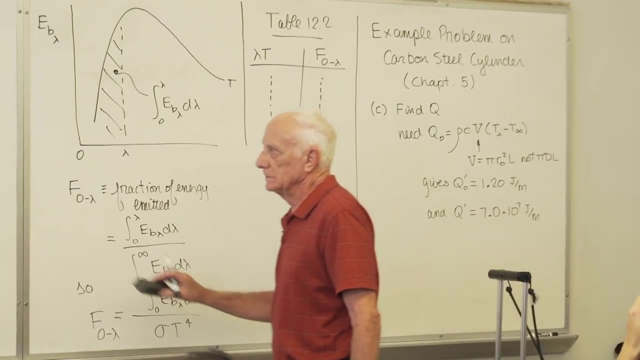 Once I know that- oh, I know this guy right here, This guy right here is Sigma t to the fourth, I'll put that down here. There, it is down there. So the table is available to do that calculation. Now I'll take one more case. 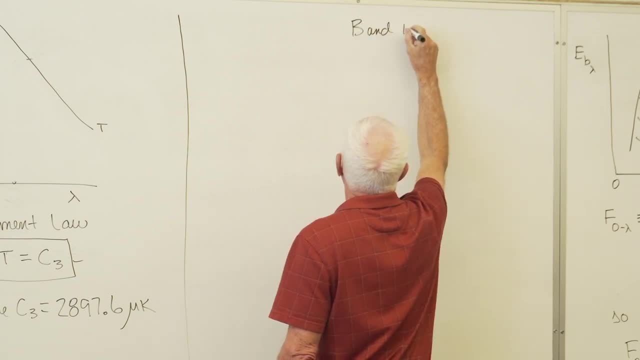 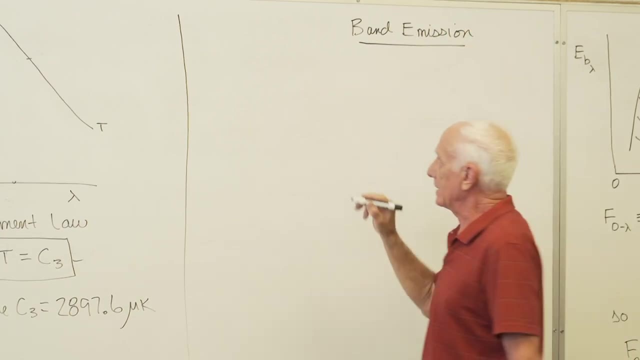 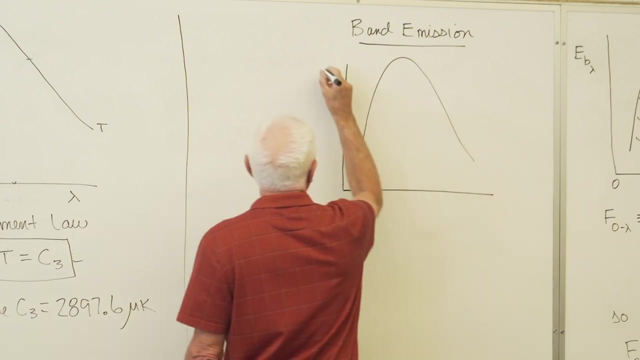 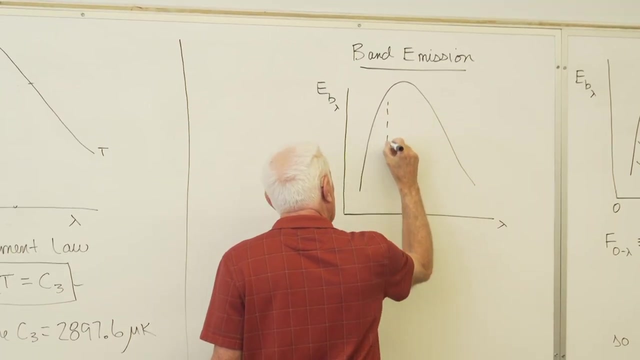 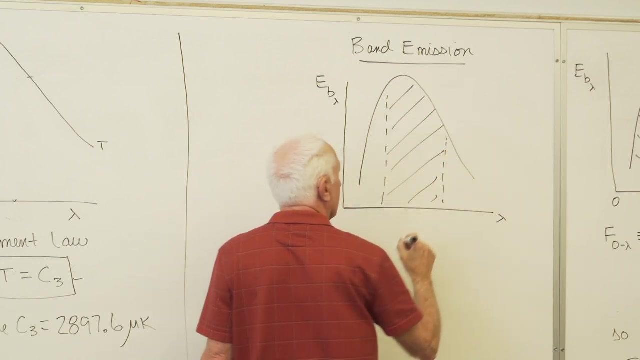 I'll take one more case. I'll take one more case Now. I'll take one more case Now. I'll take one more case. Now, I'll take one more case. Somebody said: well, you know what? I want to find out how much energy is contained in this area. 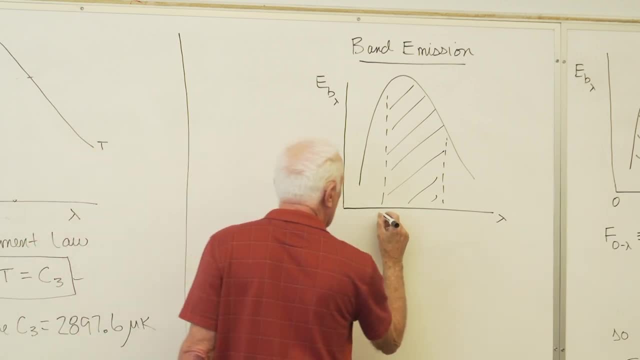 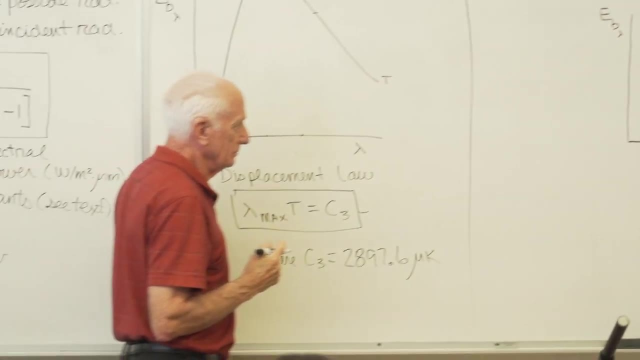 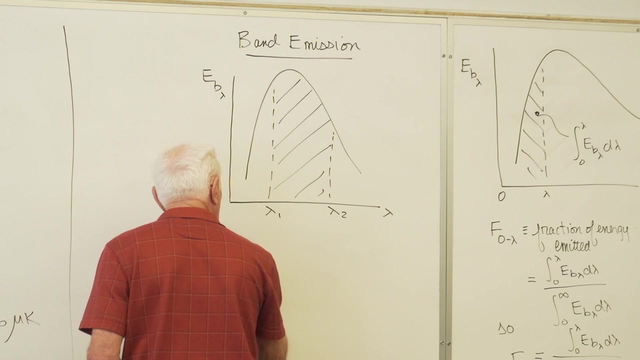 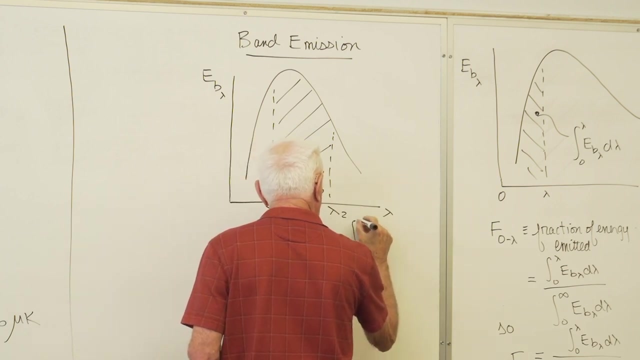 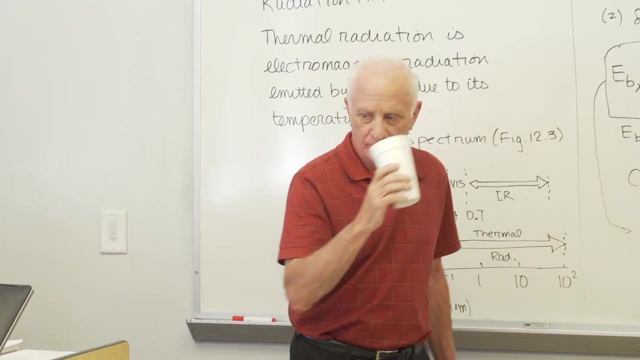 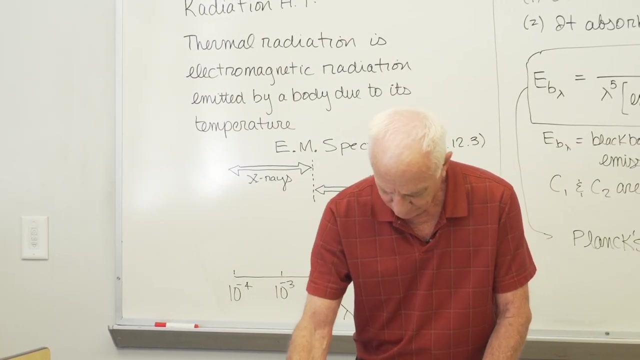 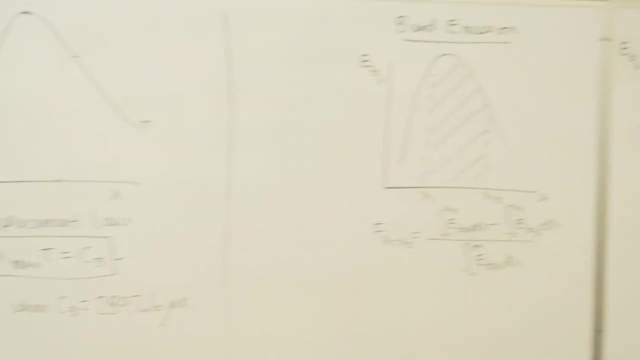 That's a band between wavelengths Lambda one and Lambda two. That's a band. We call that the band emission, So I'll write that out then. The fraction of energy contained between wavelengths Lambda one and Lambda two. The fraction of energy contained between wavelengths Lambda one and Lambda two. 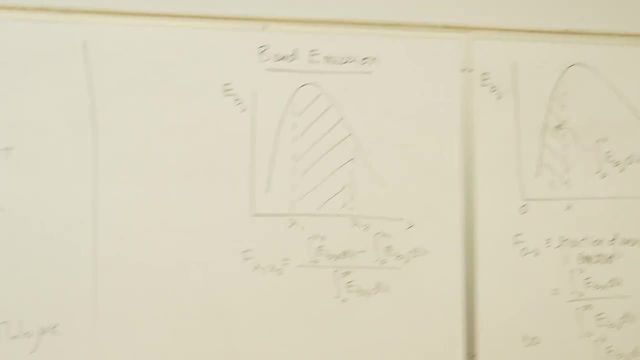 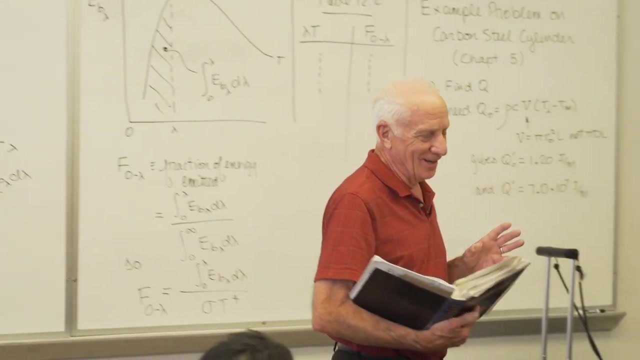 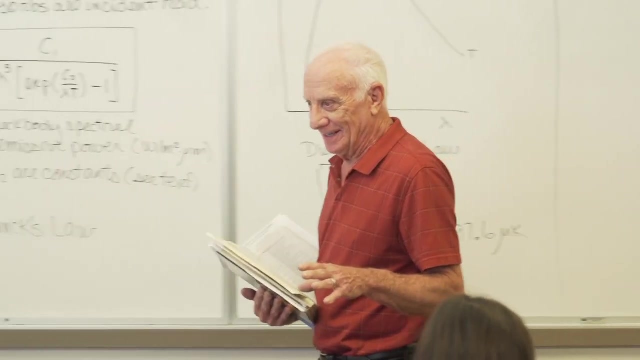 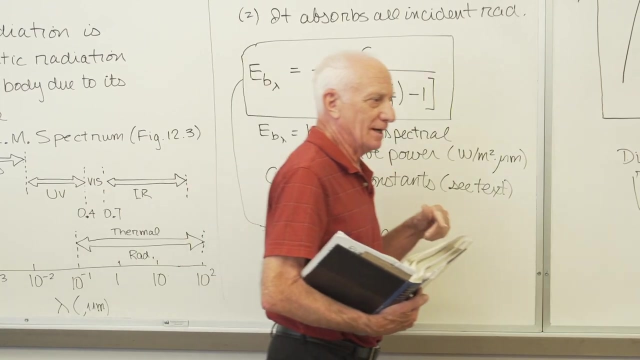 I'll proofread. Radiation in general is very vocabulary intensive. You have to understand the language of radiation or you're going to be in deep trouble. This chapter contains multiple words: The word spectral, spectral emissive power, irradiation, radiosity, specular. 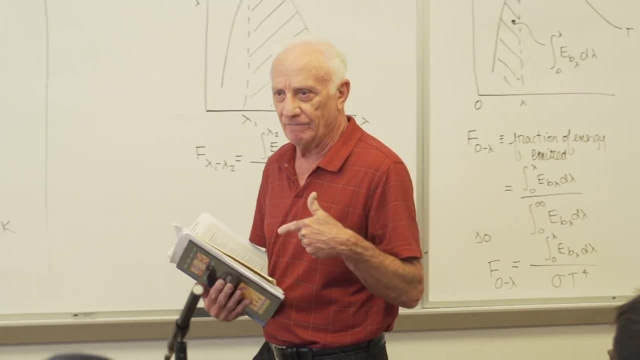 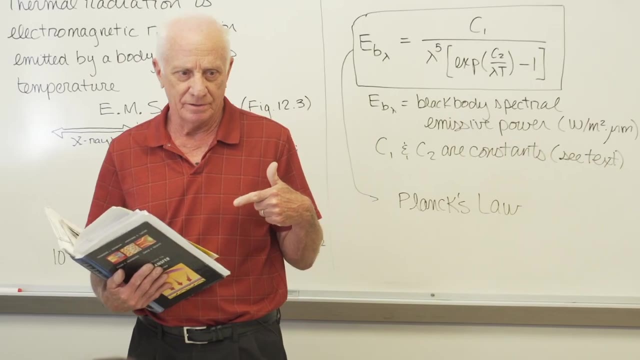 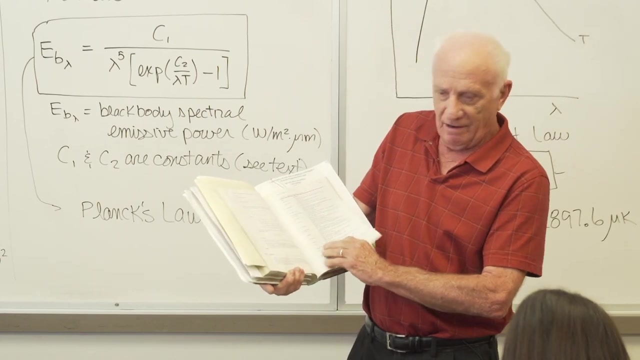 sounds like spectral. No, it's different. There's a ton of different words that mean something. It's hard to solve a problem in radiation unless you understand the language. Our authors have been very good. End of the chapter. a whole page. 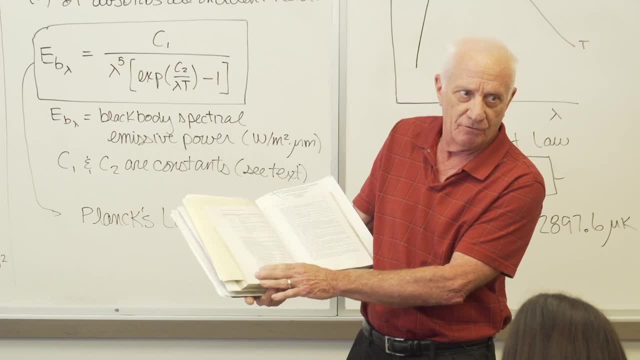 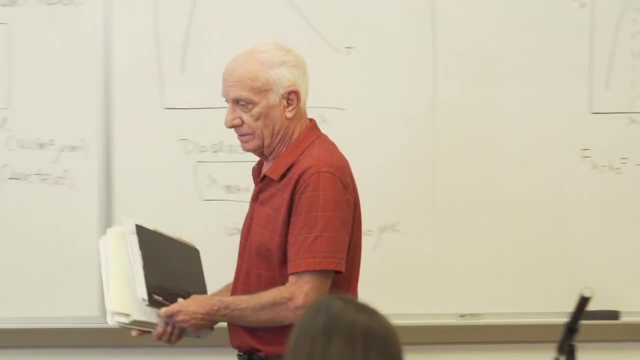 of definitions of words. half a page of definitions of words. So if you ever say, well, what does that word mean? There it is the end of the chapter. it's there. Now let's go back to here again. 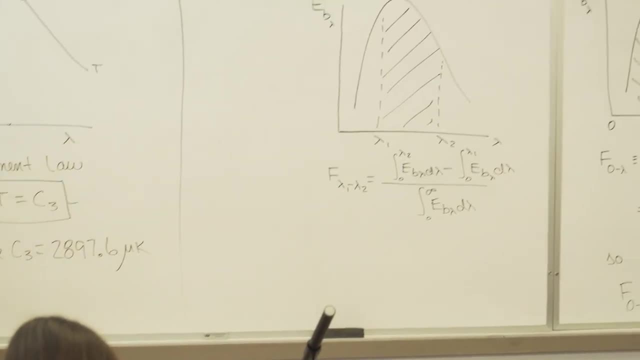 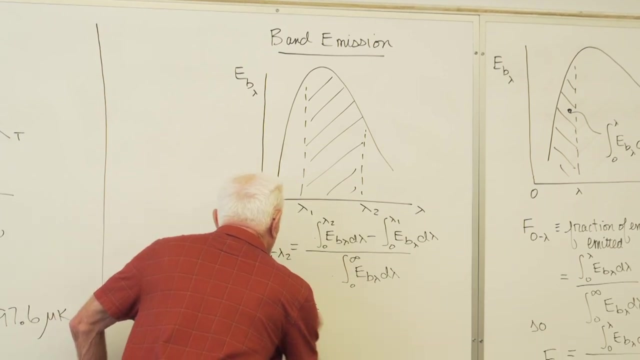 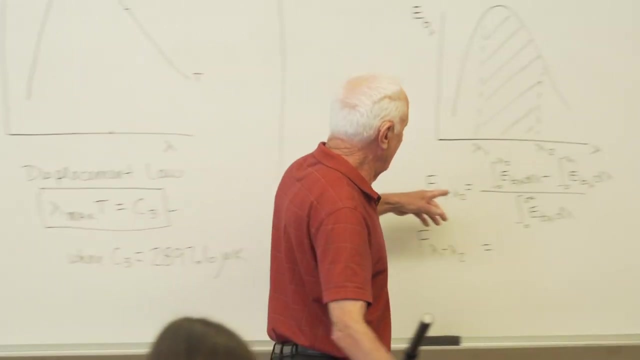 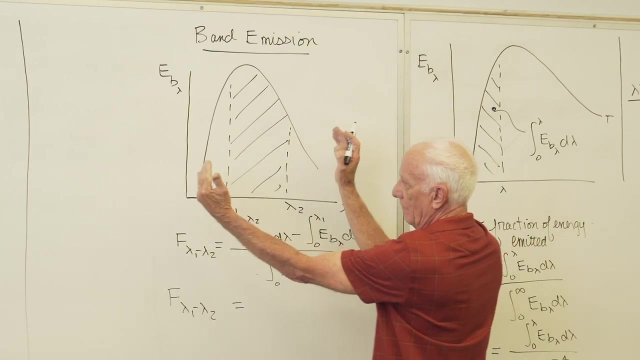 So band emission, what is this? divided by that, That's equal. by the way. let me mention first of all this numerator. What am I doing here? You can see, I'm taking the area under the curve from wavelengths of zero to Lambda two. 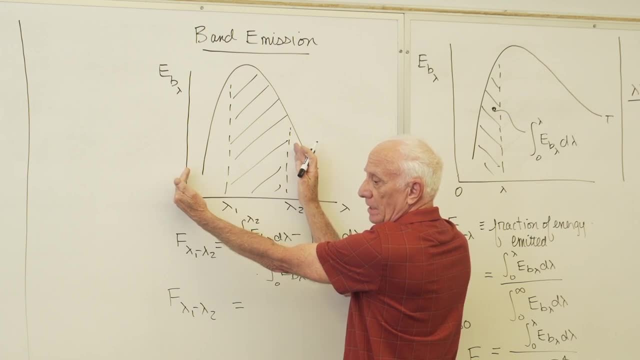 where my two hands are Subtracting, the area under the curve, where my two hands are. What am I left with This? the band, That's what I'm doing right here. Divide by this guy. So take this. divided by this. 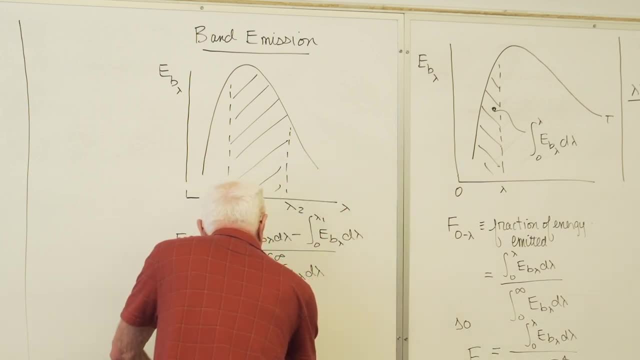 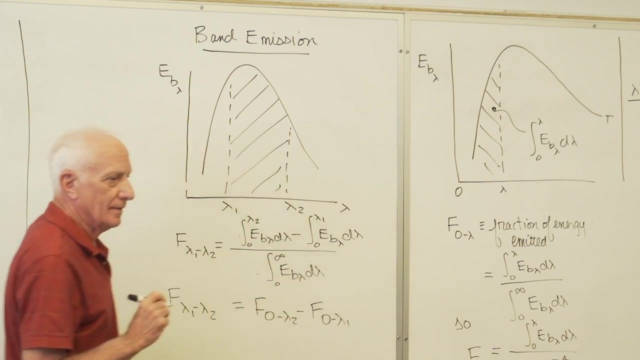 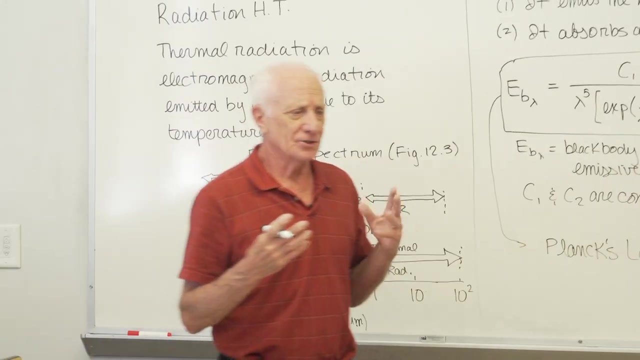 minus this, divided by this, Fraction zero- Lambda two, minus fraction zero- Lambda one. That's what we do. in the case of this, It's a band emission. Sometimes band emission could be important, like solar cells only respond to certain wavelengths, So maybe you want to know what fraction of 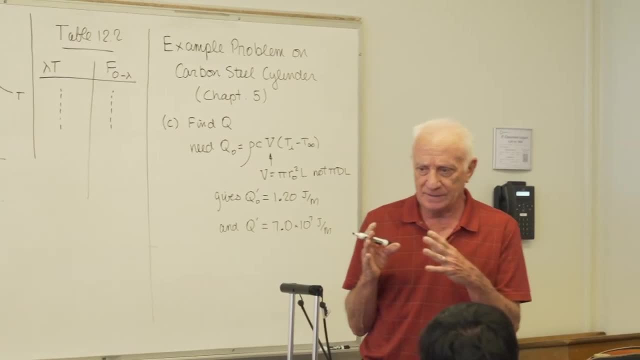 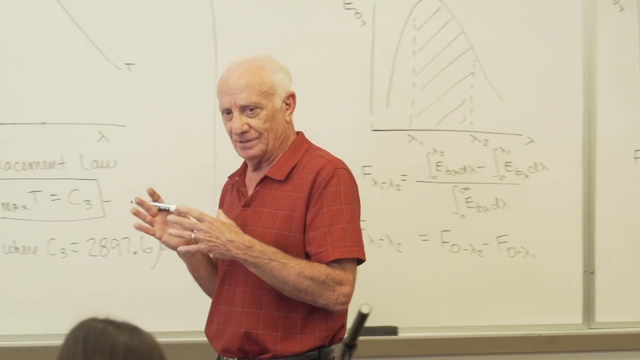 the sun's energy are contained between two wavelengths, because that's where my solar cell generates power. Okay, You're concerned about band emission then. So there are many places in the real engineering world where we're concerned about band emission Question? Yes, sir. 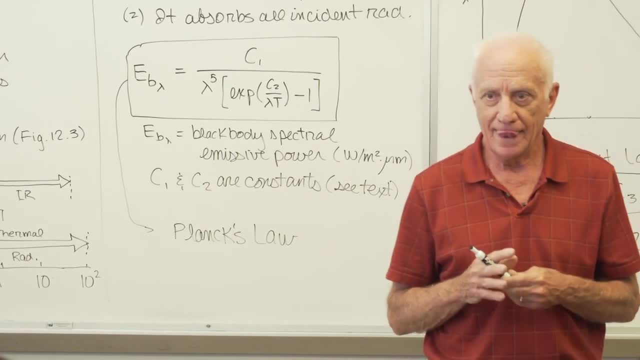 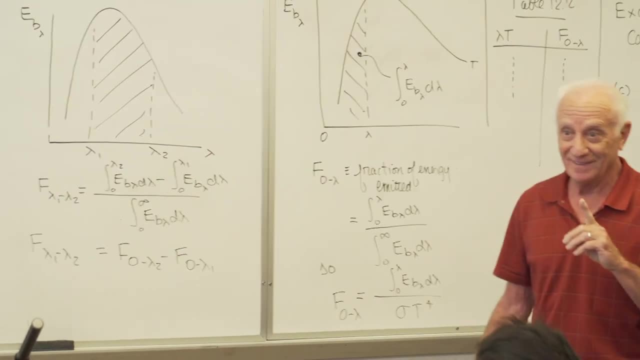 Why can't you do, or can you do, the integral from Lambda one to Lambda two? Okay, You can Do. you want to do that by hand? or do you want to go to a table? Don't want to do it by hand. 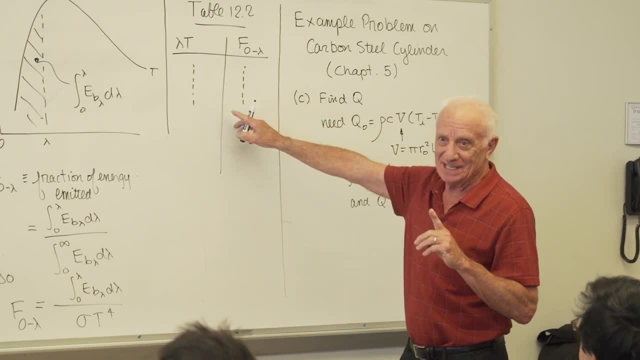 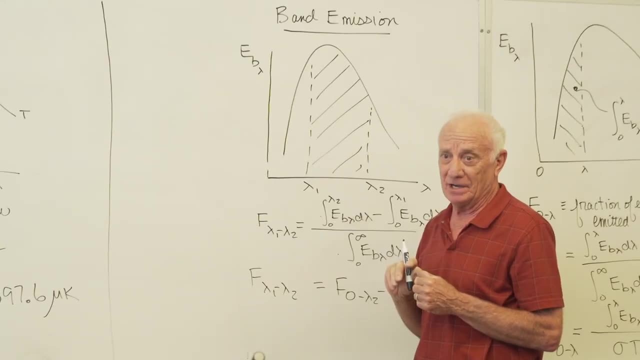 Only this table is done for you. This is the easy way out. Of course it's integral period here. But where do you find that integral? Nowhere in the book. But can you find it? Oh yeah, you can integrate it. 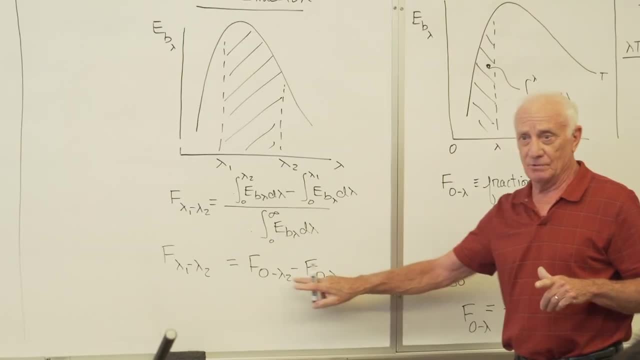 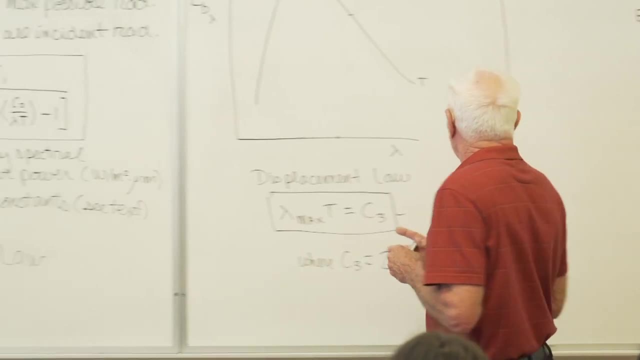 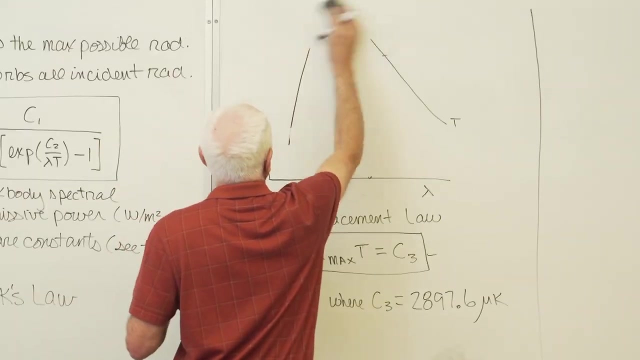 But it's much easier to do it that way, where all you do is subtract two things from the table rather than do the real calculus integration. Okay, So band emission using table 12.2.. All right, So let's look at a problem then. 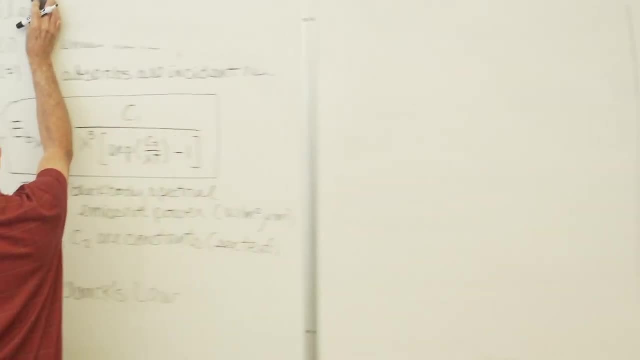 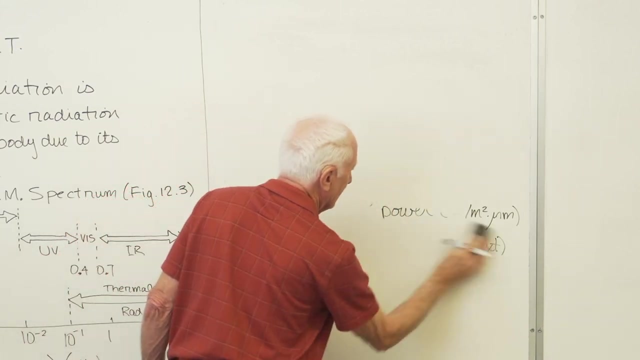 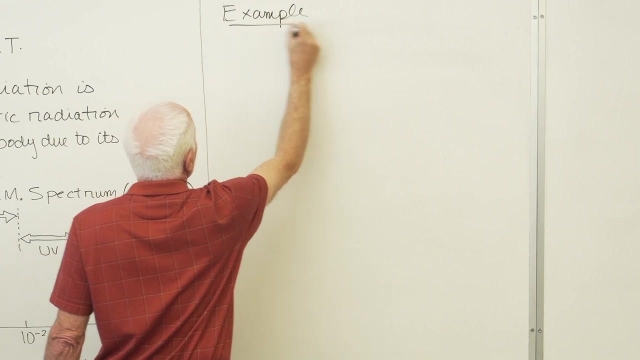 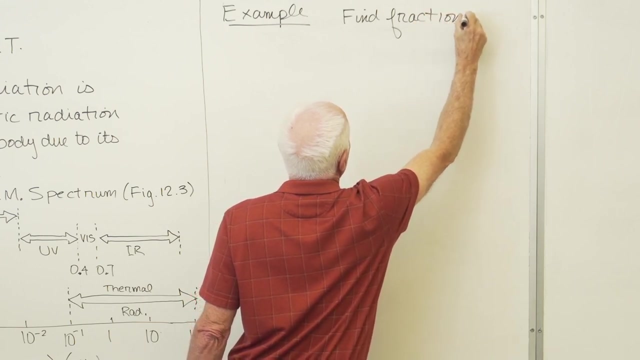 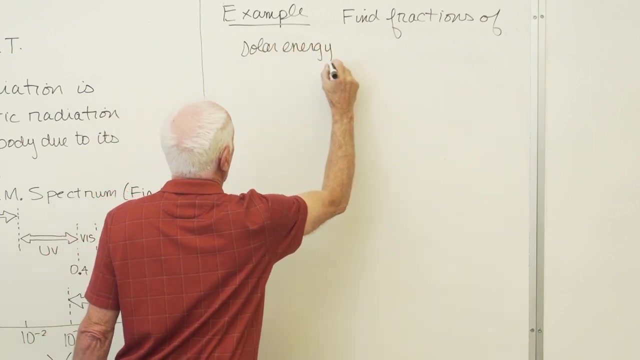 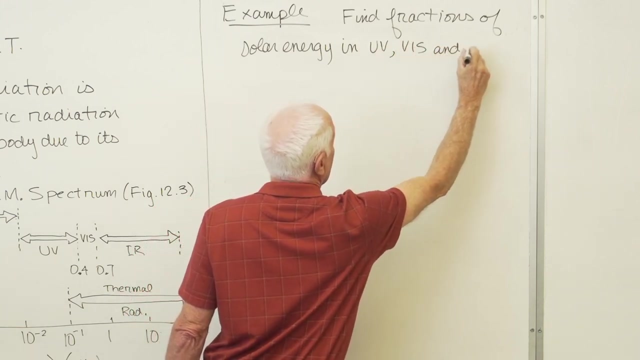 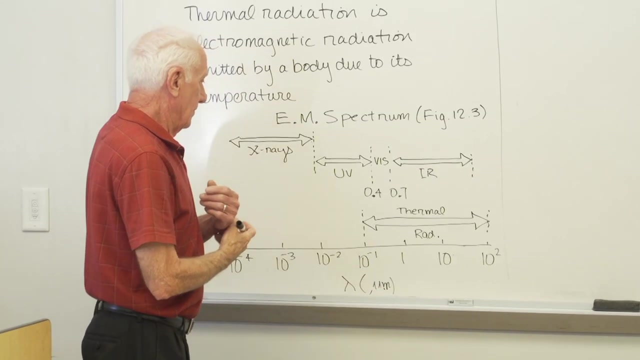 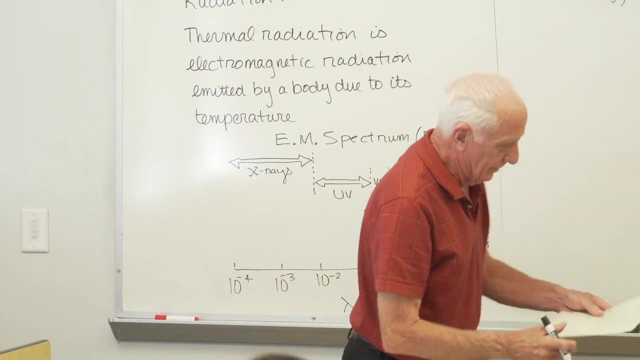 We're going to take the solar spectrum outside the Earth's atmosphere, for instance. So example: find the fractions of solar energy in ultra-violet, visible and infrared regions of the spectrum down here, All right. So let's first of all write down what my 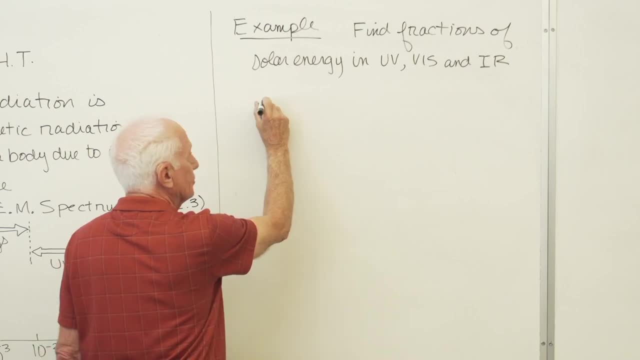 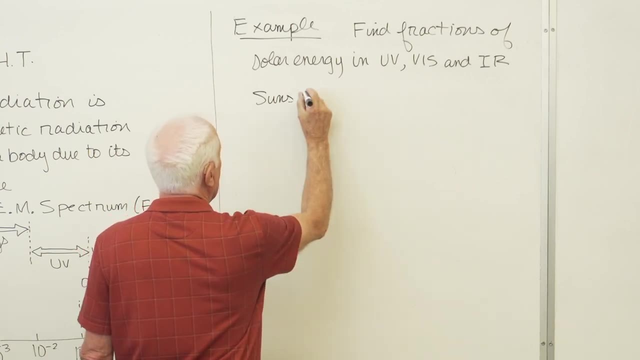 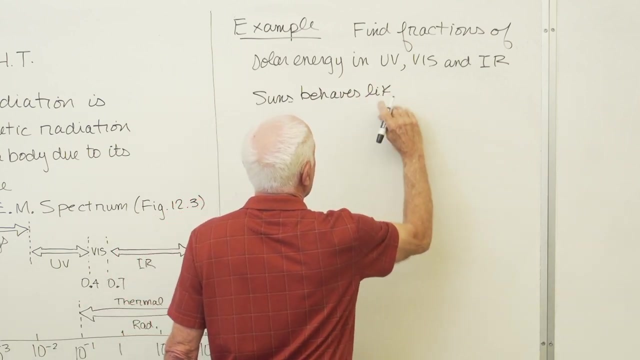 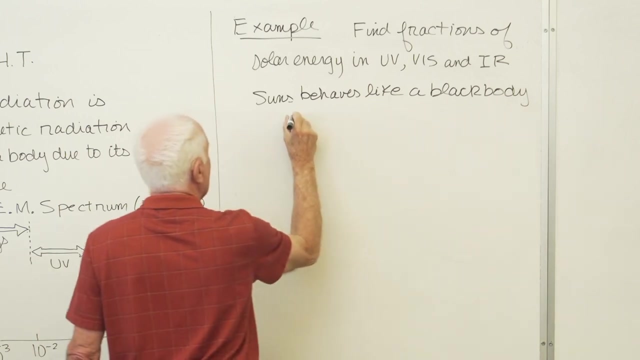 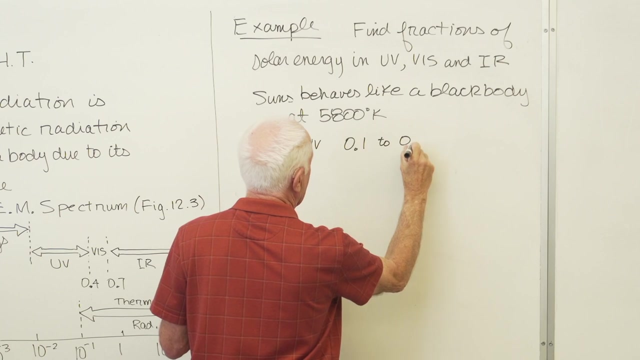 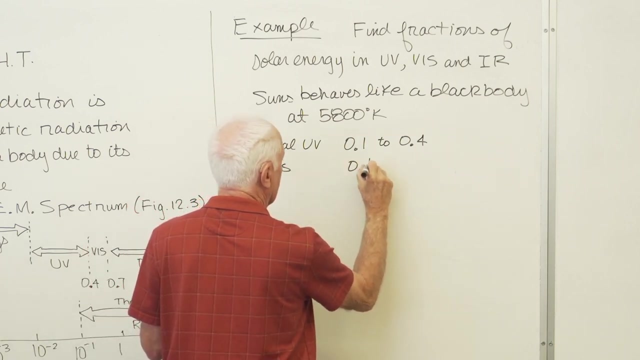 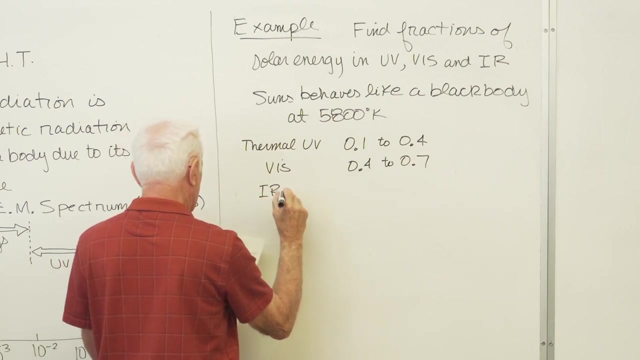 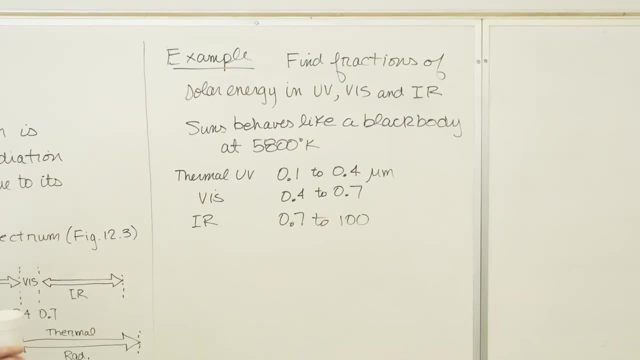 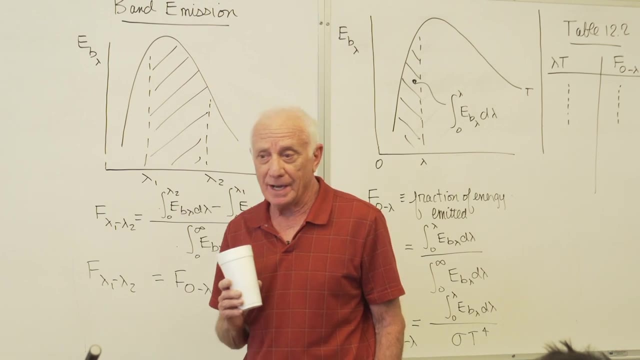 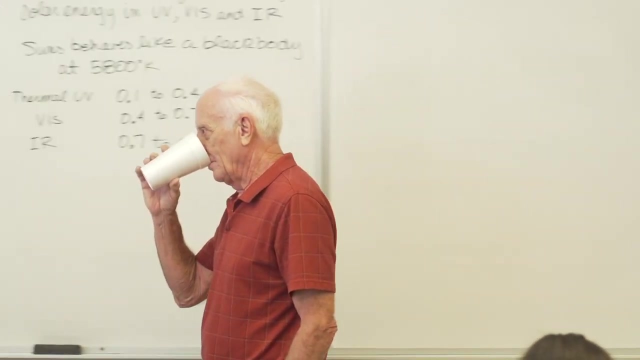 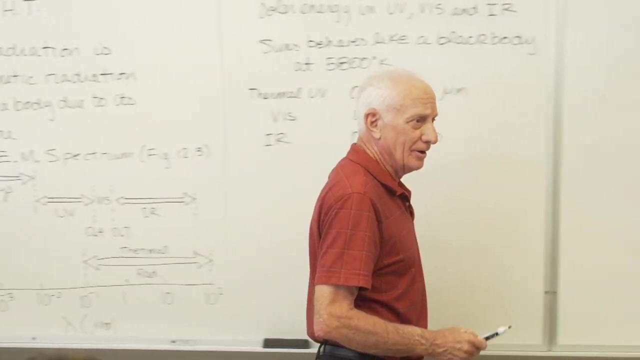 we treat solar radiation, radiation as if it came from the sun, which behaves like a black body at an equivalent temperature of 5,800 Kelvin. You say, well, did I miss something? They send a probe on the sun's surface and record the temperature. 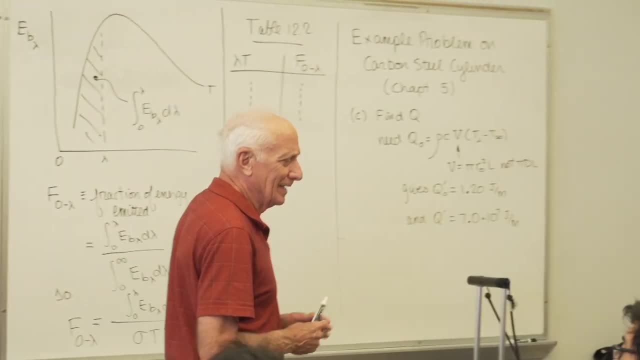 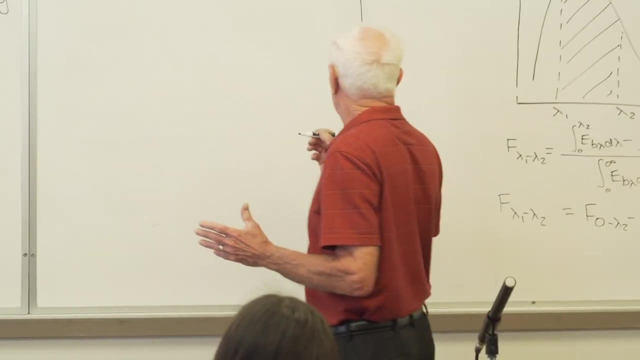 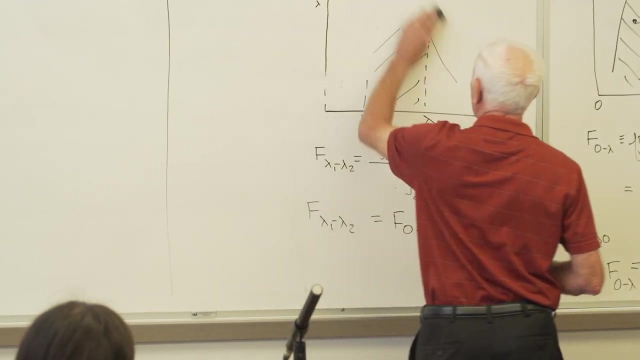 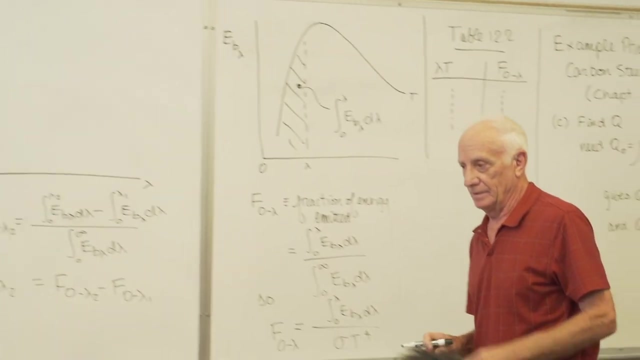 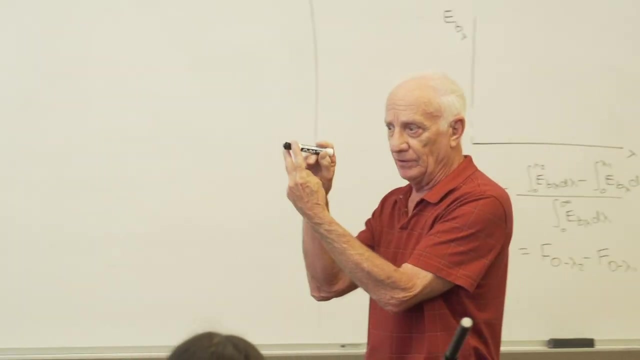 I don't recall that. No, I don't think so. So how do they get that temperature? Well, one way would be. one way would be: they send a probe up on a spacecraft satellite point a thermal detector to the sun with a certain wavelength filter on it. 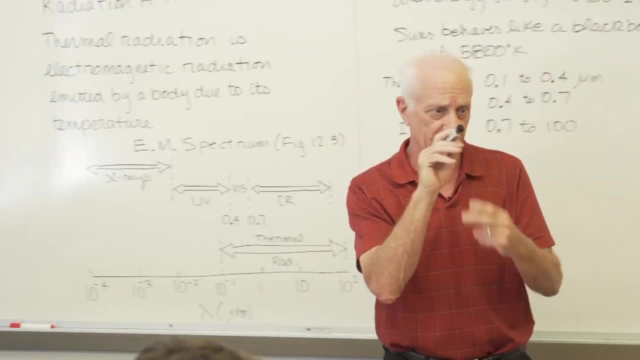 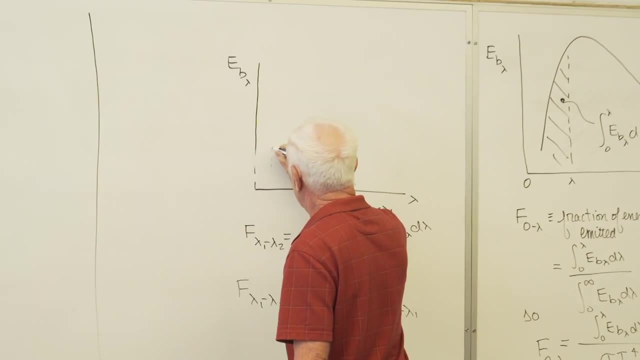 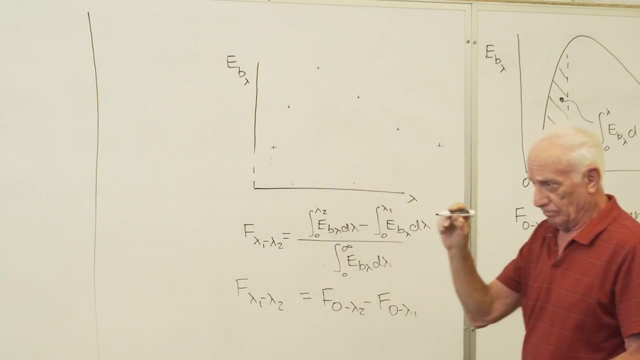 wavelength filter, so only certain wavelengths are allowed to come into this sensor. So they use different wavelength filters and they say, okay, this is what we get. That's what we get when we put different filters in here. So I'm going to connect this guy. 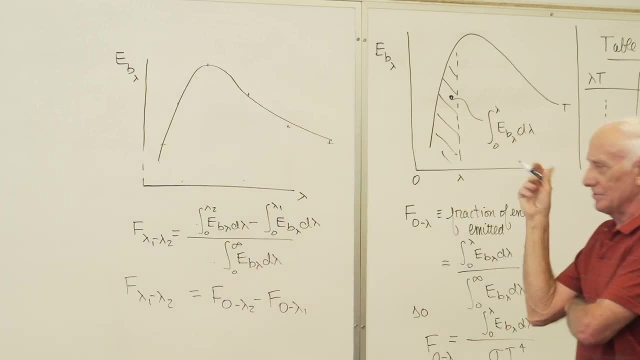 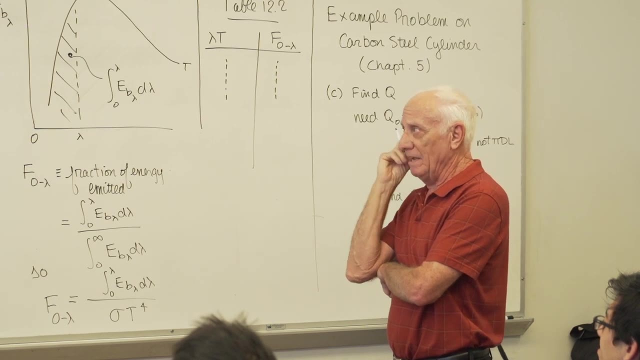 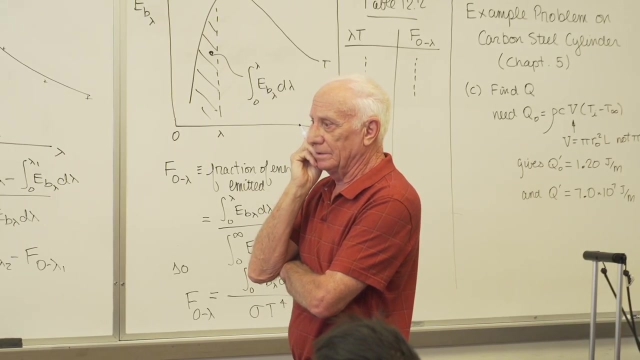 I say, hey, you know what That looks? a lot like the shape of that black body curve that I saw in the textbook. I think the sun might behave like a black body. Okay, good, I'm going to assume the sun is like its equivalent temperatures. 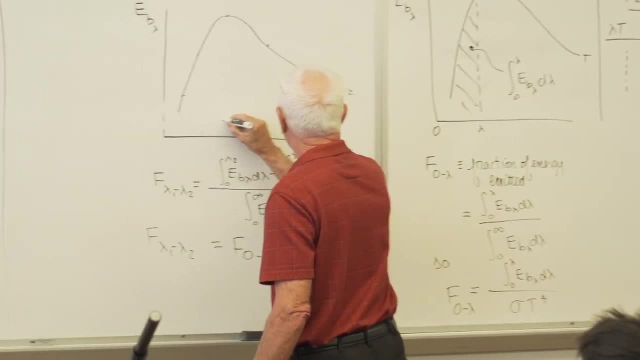 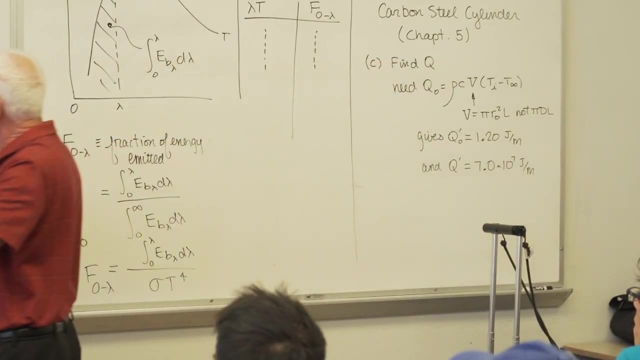 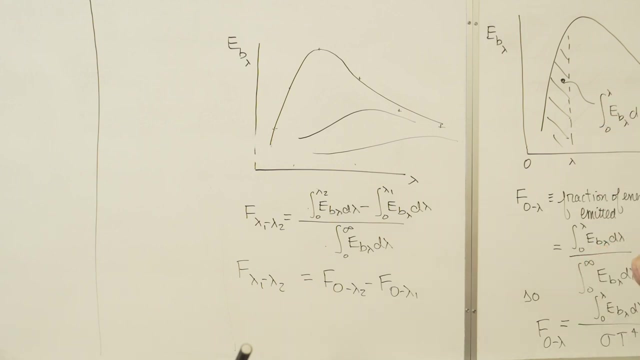 300 Kelvin room temperature. No room temperature. No, not even close. I'm going to guess the sun's temperature is 1,000 Kelvin. getting there, I'm going to guess the sun's temperature: the sun's temperature is 10,000 Kelvin. 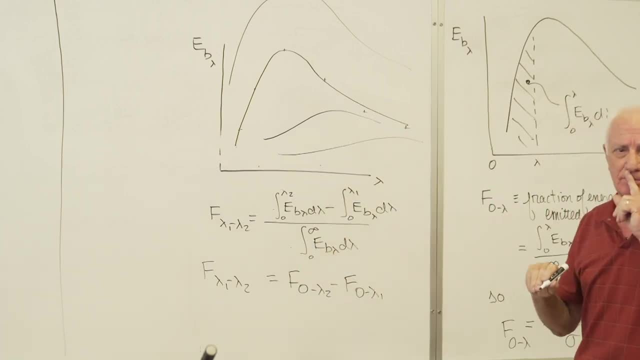 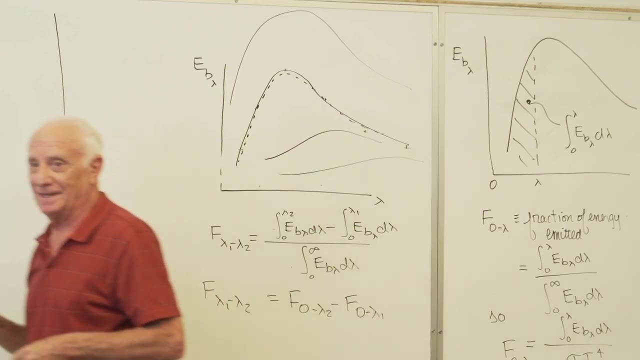 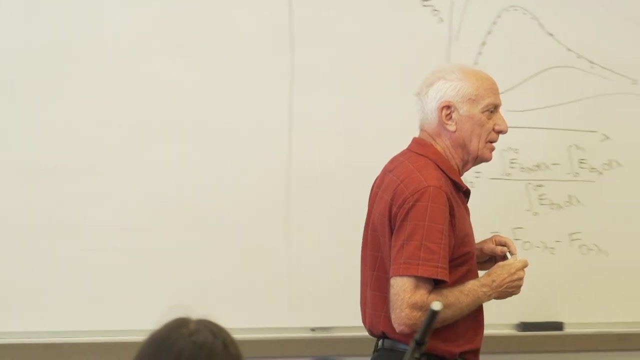 Oh, no, no, no, no, no. I'm going to guess the sun's temperature is 5,800.. Say whoa, I got it, I got it. My best guess now is the sun is behaving as a black body whose temperature is 5,800. 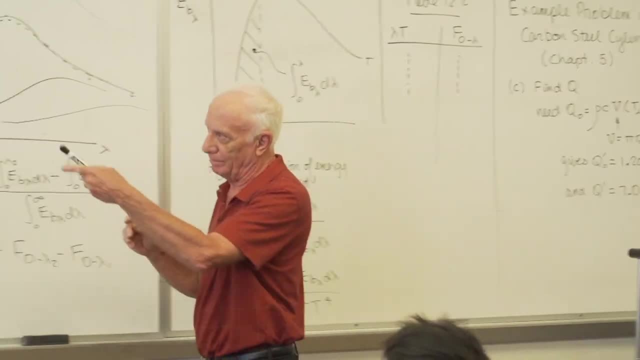 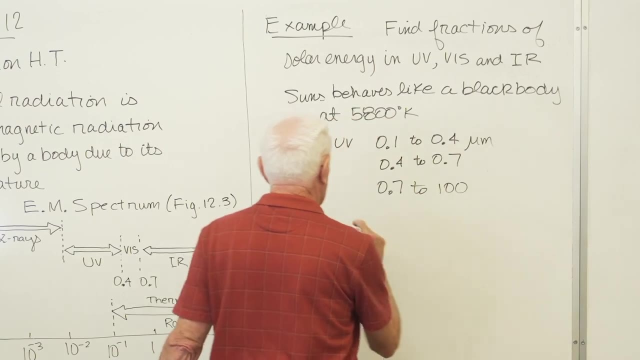 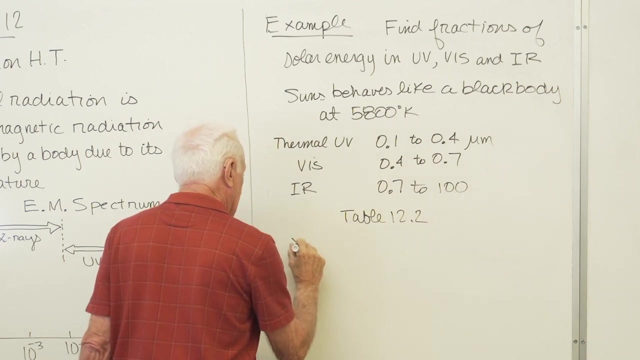 Good, That's what we're going to use in this class from now on. Okay, back over here. So here we go. That's where that came from- To use that table, table 12-2.. Okay, Lambda-1t equal Lambda-1,. 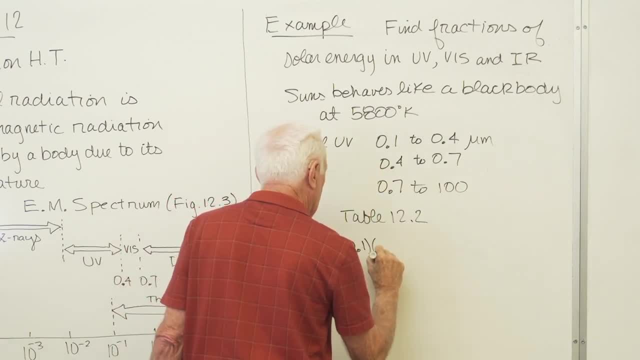 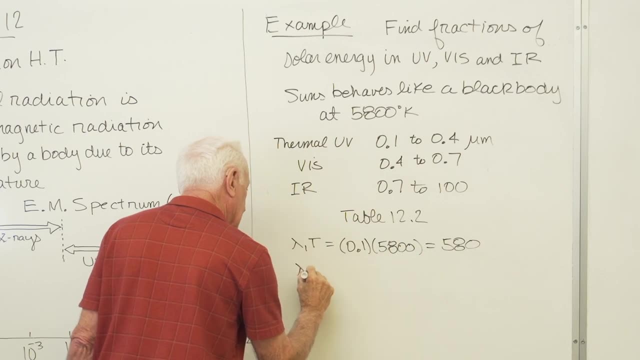 one-tenth Temperature: 5,800, 580.. Lambda-2t- I put them all down. Lambda-3t, Lambda-4t, 580.. Lambda-3t, slide 2, lambda-4.. Thank you. 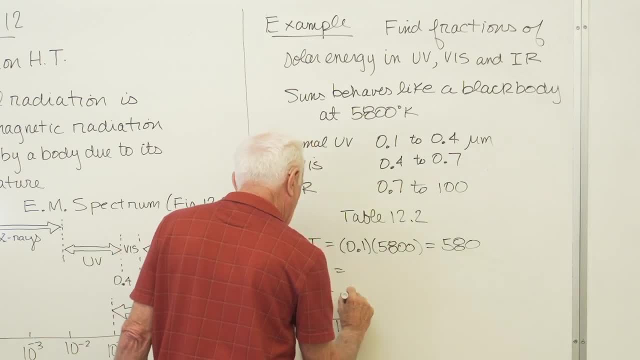 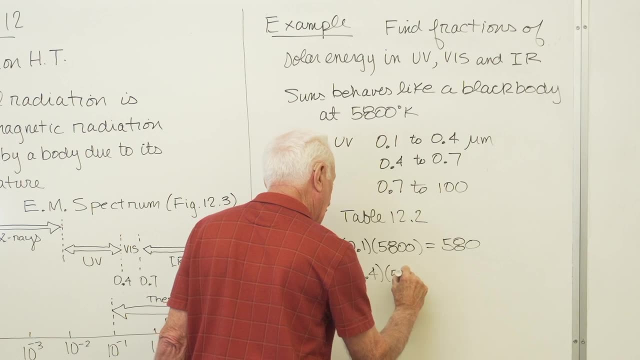 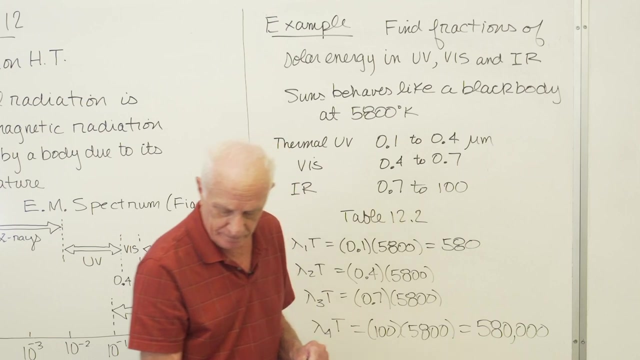 Lambda-3t be four-tenths 5,800.. Seven-tenths 5,800.. 100 times 5,800, 580,000.. 23,, 20, and 40, 60.. 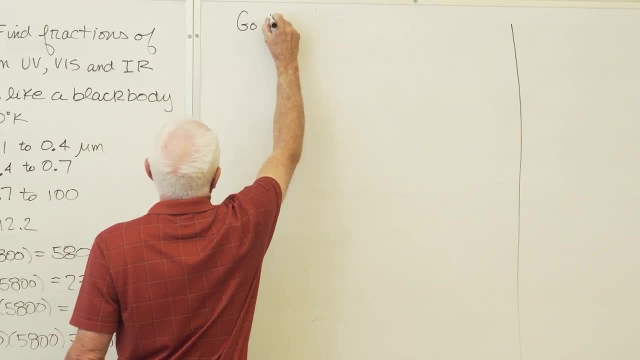 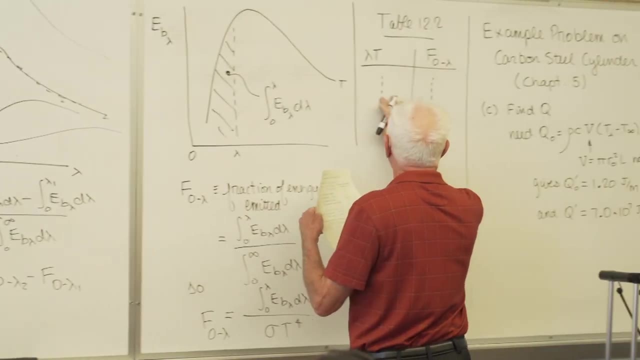 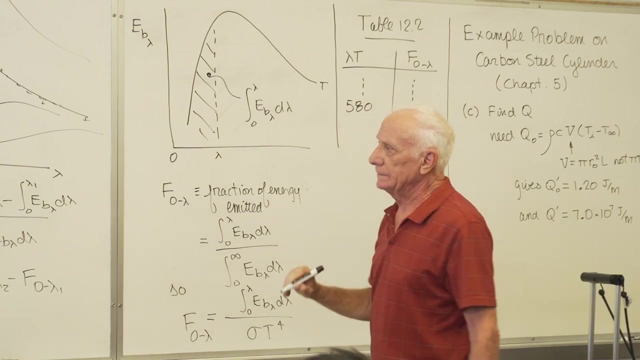 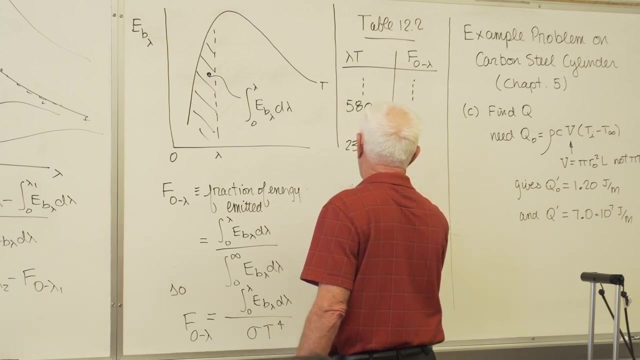 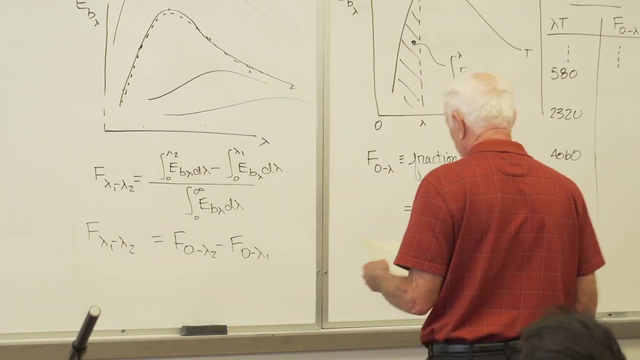 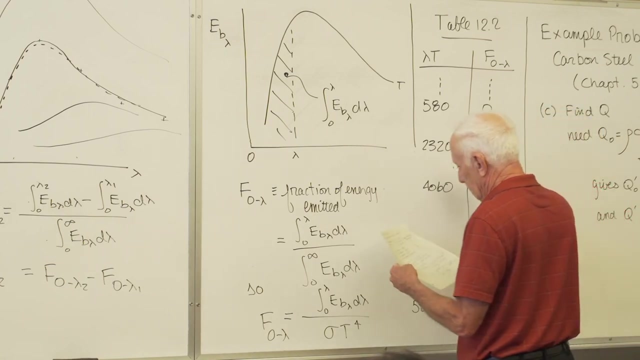 Now go to table My first lambda, t 580.. Second one: 23,, 20, and 40,, 60, and then, way down here, 580,000.. Fraction 580,: 0,, 23,, 20.. 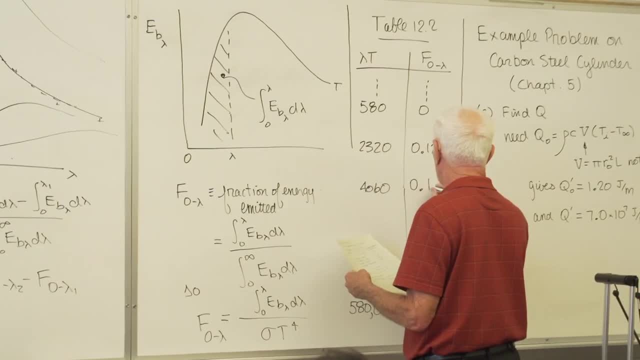 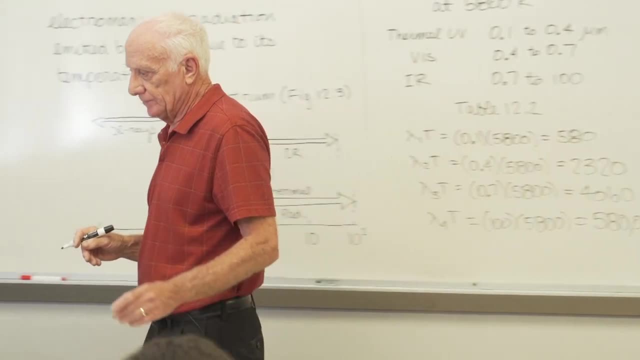 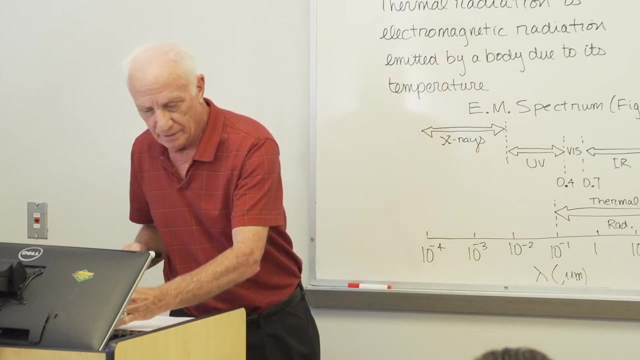 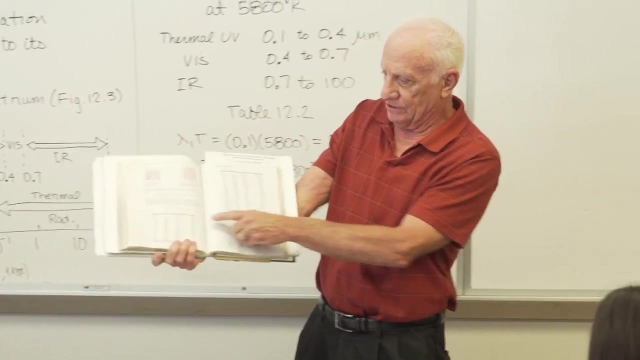 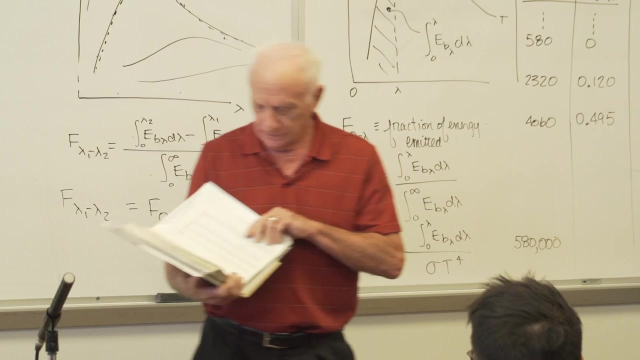 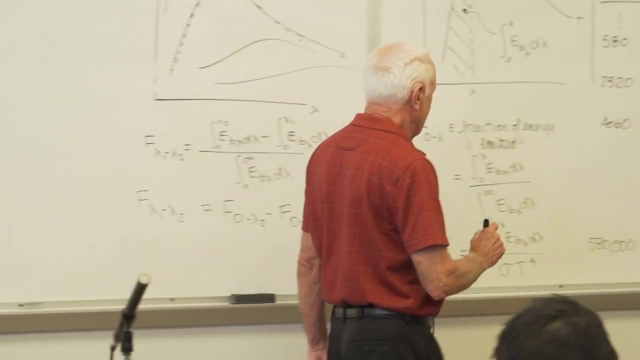 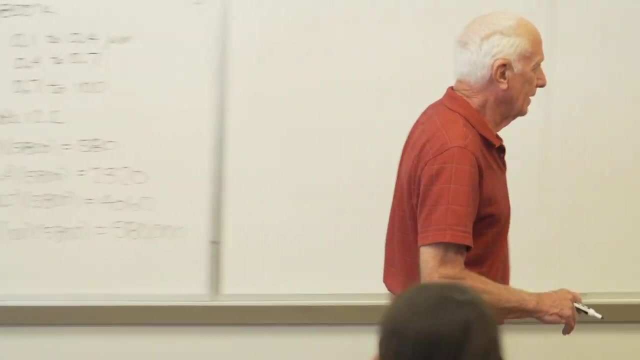 40, 60. Almost there. Table's really long in the book. There it is, Starts on one page, ends up over here, big table, The last table entry 100,000?? Make sure, Yep, 100,000.. Last table entry is 100,000. 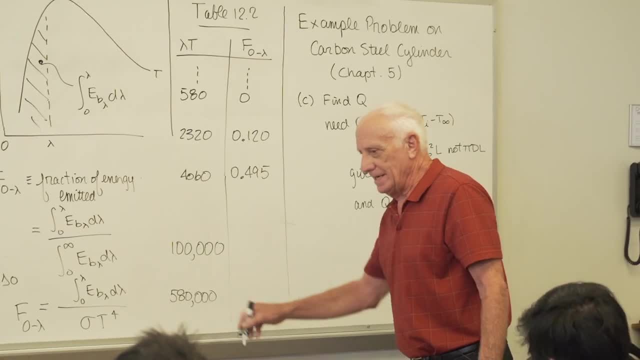 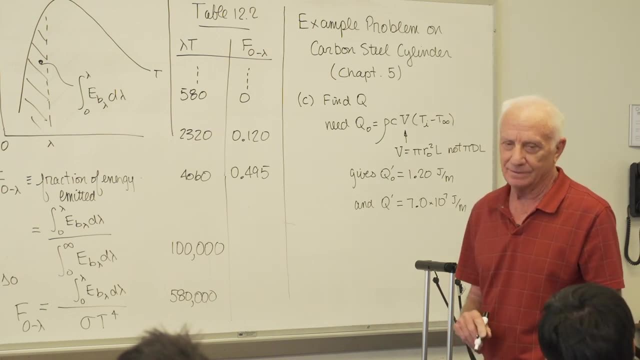 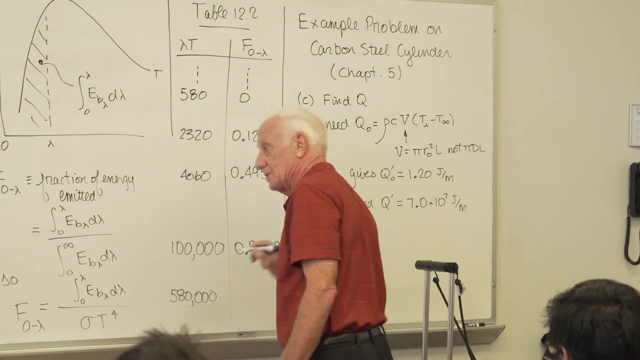 That's not going to work. I need 580,000.. The table doesn't give me that answer. It's not even close to it. Yes, it does 100,000,. I'm going to extrapolate. Sometimes extrapolation is good. 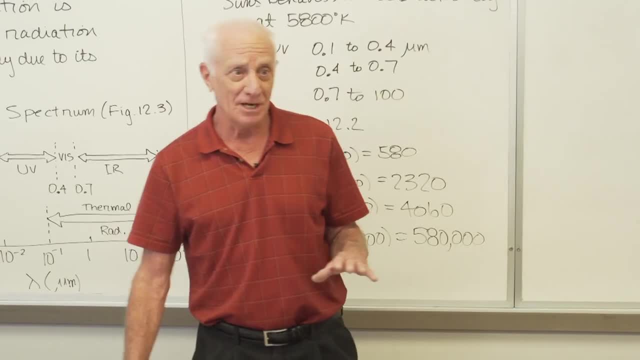 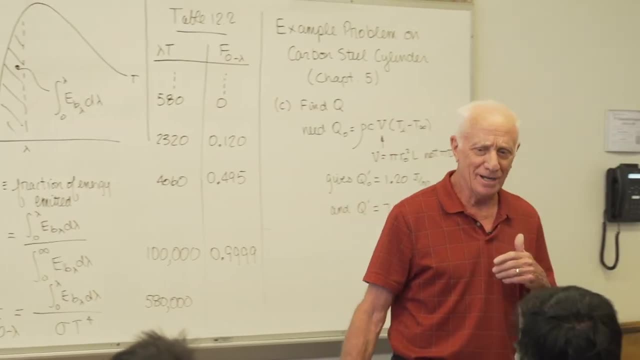 Sometimes it's bad. In this case, extrapolation is fine. I'm going to round it off to 1.00.. Of course you will. Why not If it's 0.9999,? guess what 580,000 is?